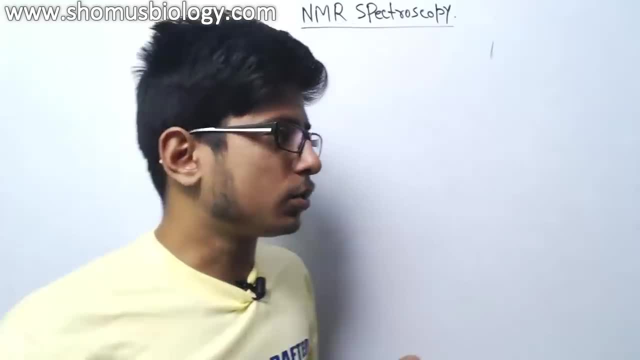 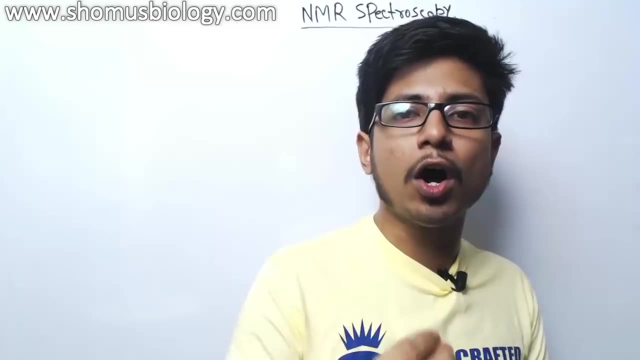 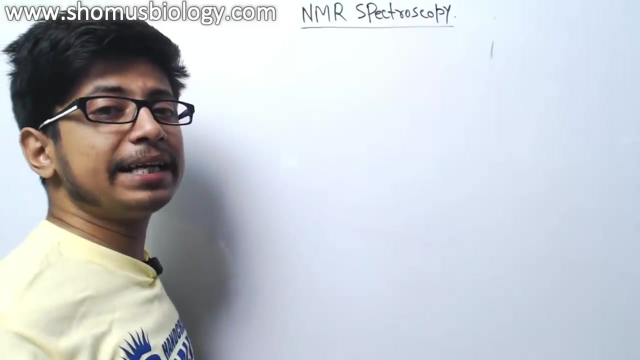 of NMR spectroscopy in this video. The first thing I want to talk about is that NMR spectroscopy exploit the idea of spinning and the, the, the feature of electron as a magnet. So what we mean normally, what we know as it says, nuclear magnetic resonance, that means all of this. 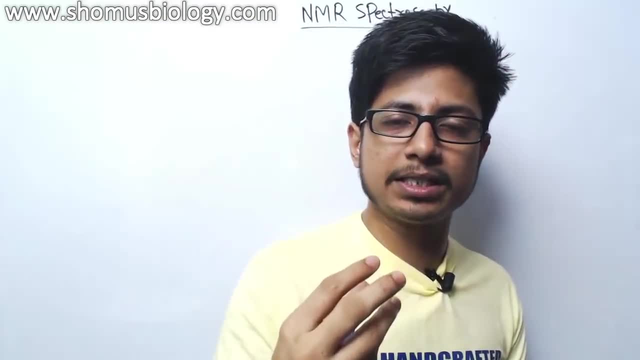 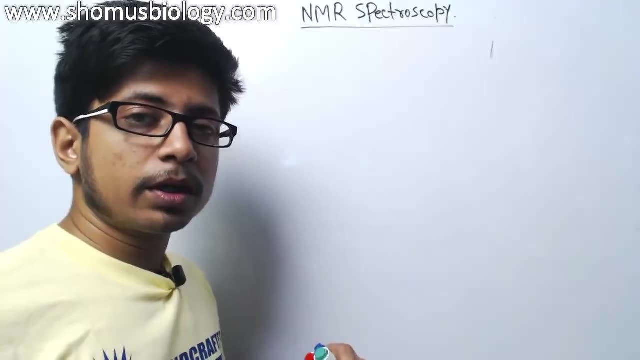 atom, they have a nucleus. we know that that atom contains a nucleus and the nucleus is surrounded by electrons. That's the idea for understanding NMR. will start to talk about the simpler form- often atoms and molecules- and go to the complex form. For example say: 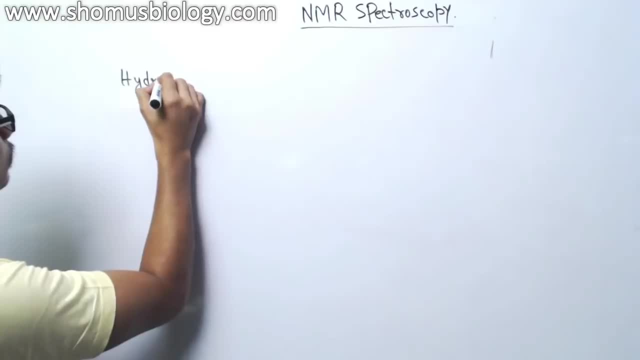 if you begin with hydrogen you can tell a very simple structure, because hydrogen mostly one proton and one electron. proton is in the middle in the nucleus and the electron is usually the nucleus and the electron is the nucleus. So there is only node in each of the four protons and one electron, only one electron. this is the control by which NMR spectroscopy, という NMR spectroscopy, helps you understand the nMR spectroscopy. I am saying No number of rectangles that are circulating in one second. So let me tell you a joke by making electoral. 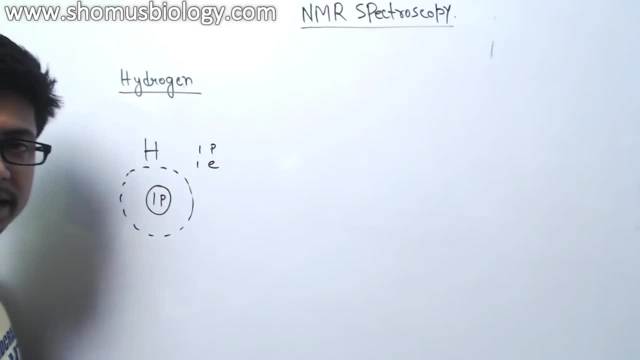 is circulating this proton, That's the idea that there's a structure of the hydrogen. Now, here in this process of NMR spectroscopy, we will see this proton playing vital role. What kind of role that this proton can spin? It can spin due to the spinning property of 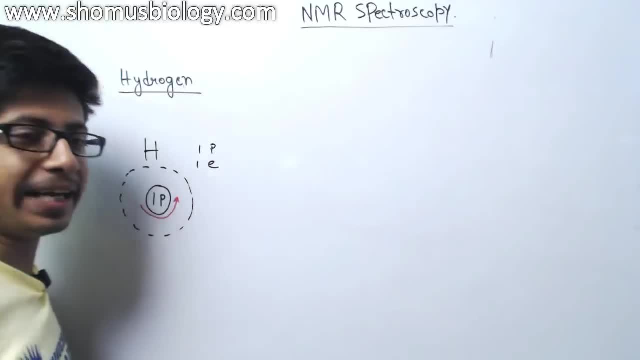 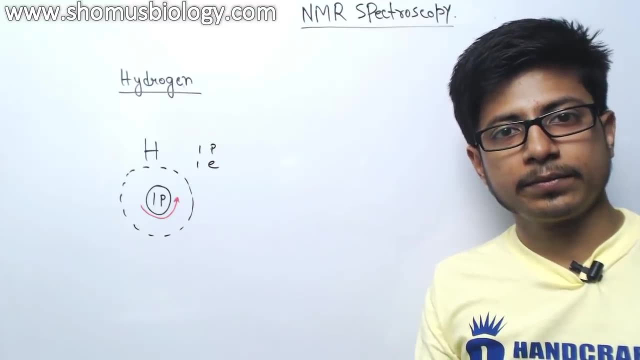 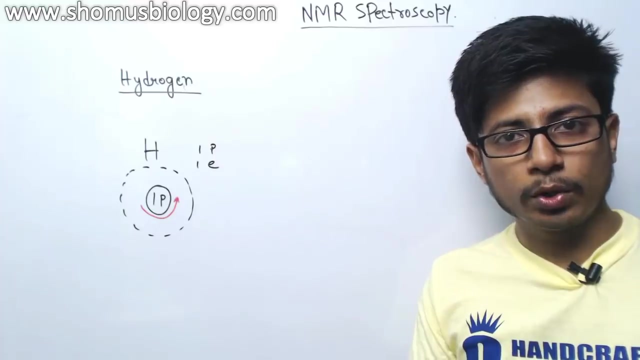 the proton, It can be like a magnet, and this is not only true for hydrogen, This is also true for many other type of atoms, For example nitrogen, carbon chlorine. all these things, they have the same property, They have the proton, and that can spin the reason for the 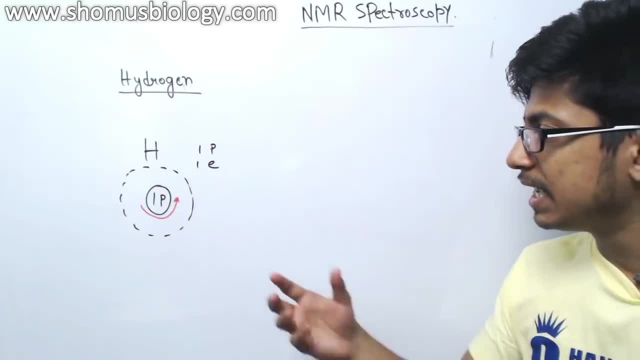 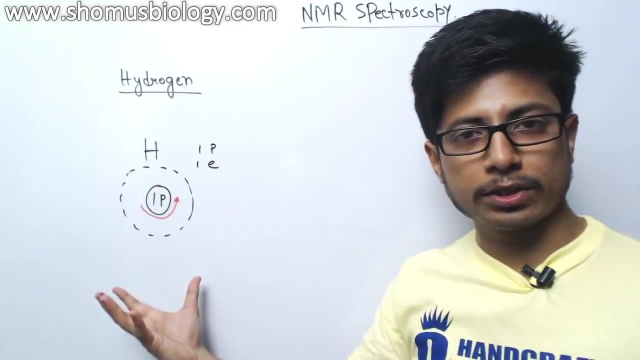 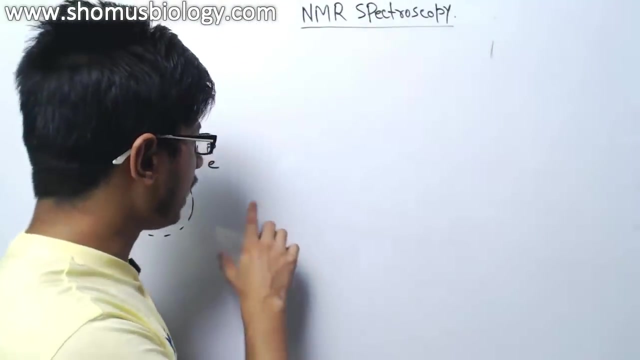 spinning The. that's the reason that this proton is spinning. due to the spin, They get the magnet. Now, for the simplicity's sake, we only take hydrogen and explain about hydrogen in the process of NMR spectroscopy. Now, as I told you, like the hydrogen can spin, So I told 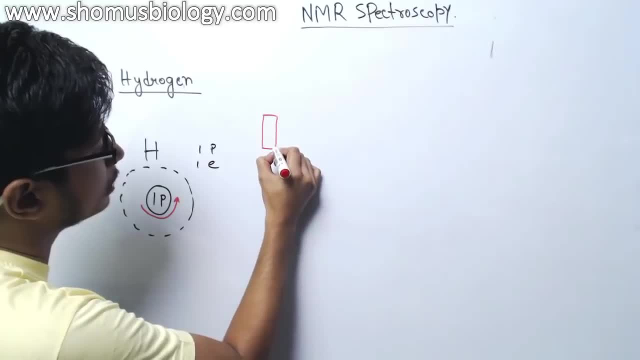 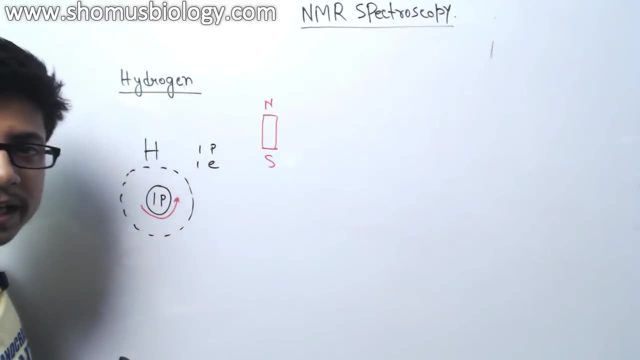 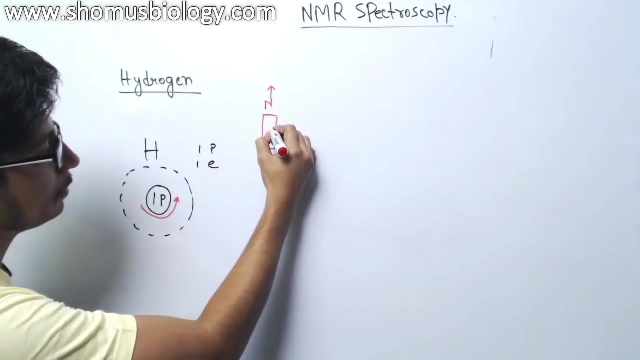 you like, it can act as a magnet. So let's assume this hydrogen acting as a magnet and if it's a magnet it obviously have a North Pole and a South Pole like a every magnet. So the North Pole like an arrow. How you designate a magnet, put an arrow to the North North, just like a. 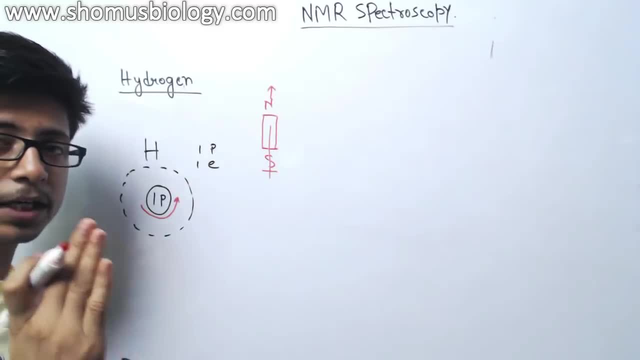 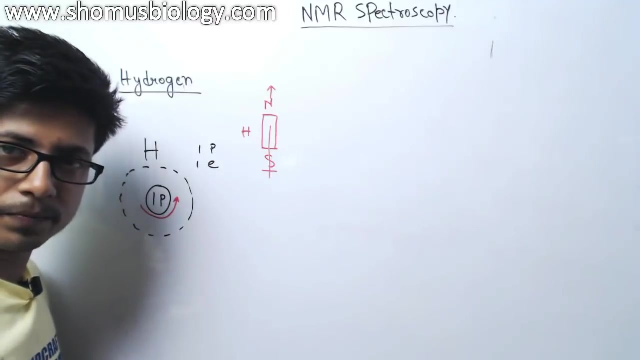 brittle representation, because that is, that is the direction. west magnet always pointed to The hydrogen. we have been like a magnet, no one thing. you should understand the magnet, The magnet close to the hydrogen, pigeon hydrogen. you put the hydrogen across to this one. Let's say we've been on hydrogen hydrogen or the방 one. you can notice. So it is you. and I put the magnet in pictures so you can see the magnet very closely exposed like this. So it is North Pole. Now one thing you need to understand: once it is a magnet, this would be a magnet close to this hydrogen. that could be another hydrogen atom, specific hydrogen atom very close to this one. This is another hydrogen atom very close to this one. Let us say we bring another hydrogen atom. 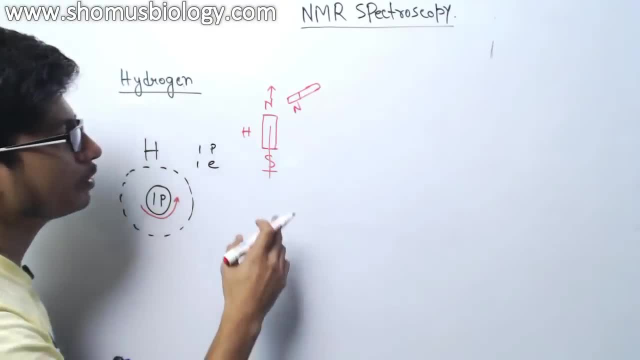 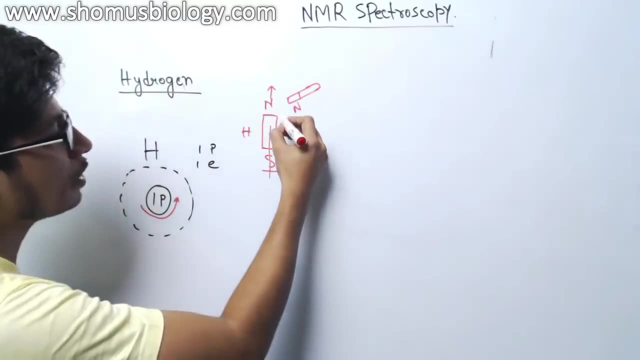 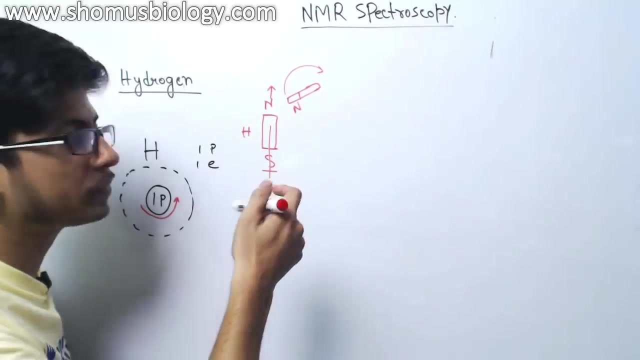 with north pole towards the north of this hydrogen. So this north north will ripple each other out, So it will try to rotate the other one in the opposite direction. It will allow the second atom to spin so that the south pole gets near to the north. So they 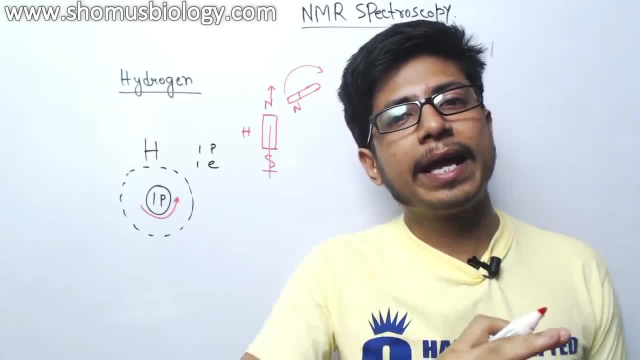 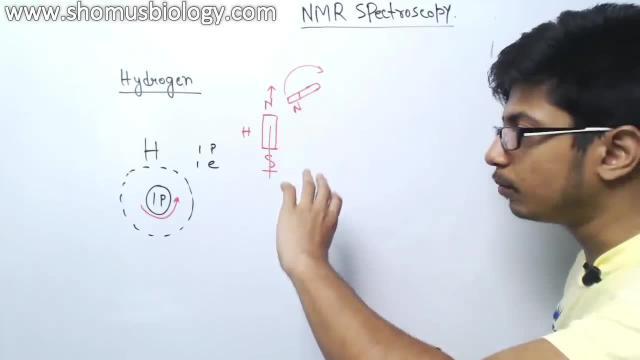 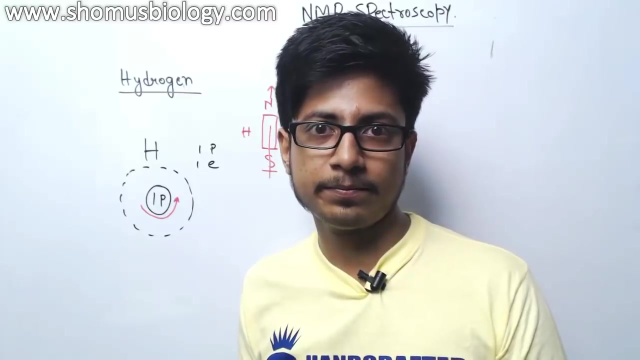 will have a rearrangement, And this is true for any magnet that we know of. And this rearrangement is really important because, after the rearrangement, whatever structure they acquire, that is known as the stable state or least energy state, That is, the most economic state, this atom. 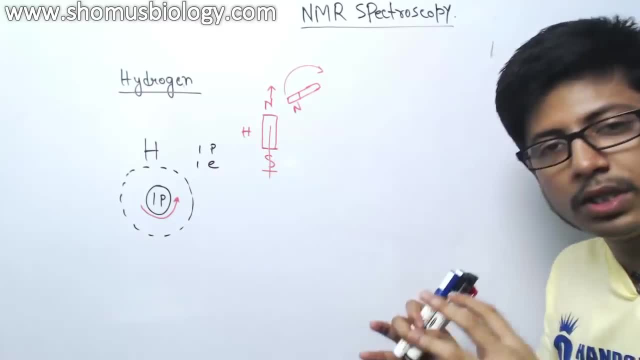 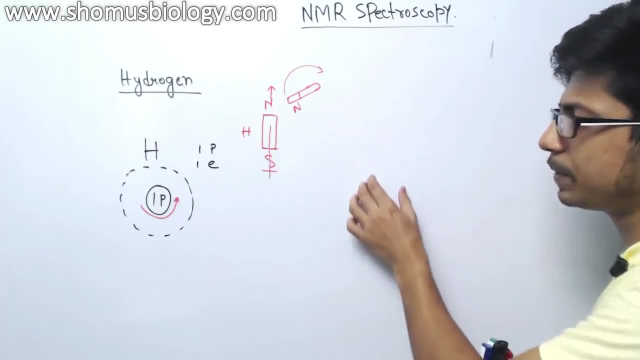 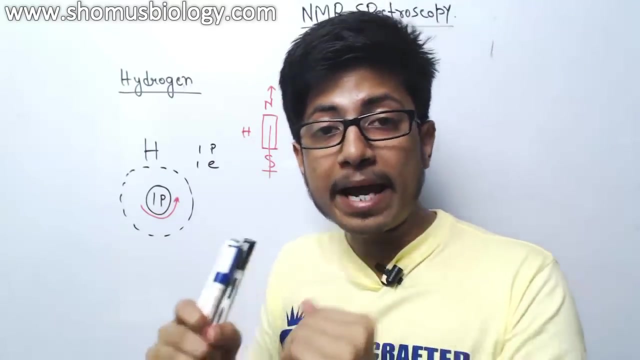 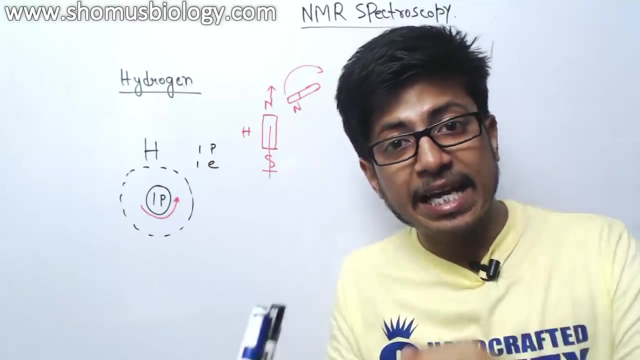 can be. So they want to be in those stable state. Now imagine the situation. This hydrogen is present And if we put some kind of magnetic field? magnetic field means we are providing a direction of north with the help of a machine that will also do the same type of effect. right, So let me? let me draw the 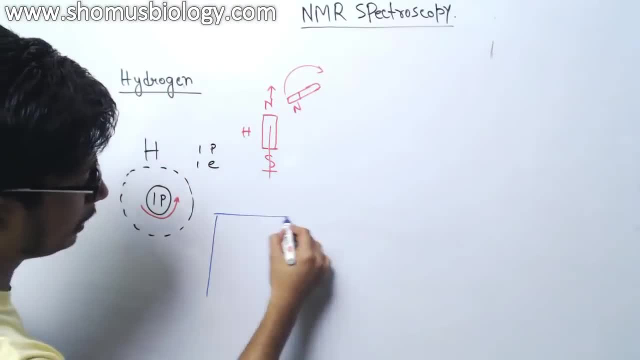 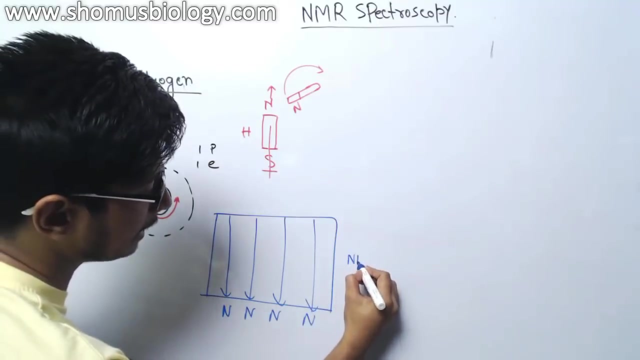 same thing here. Let's say, here in the machine we are providing this. This direction of the arrow is the field towards the north. So this is the north field And this machine is known as the NMR machine. The job of any of our machine is to create. 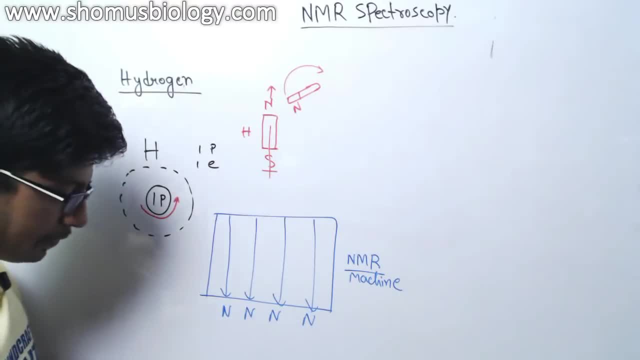 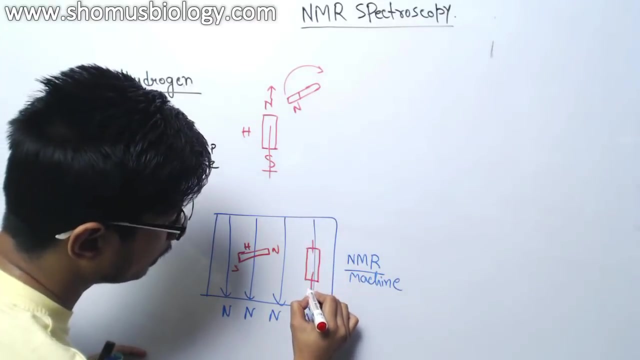 a magnetic field. As we are creating the magnetic field. what we know is that, in whatever direction that hydrogen was, let's say, this is the north, this is the south, in whatever direction it was before, Now it will be shifted to only one direction, That is, this one. So 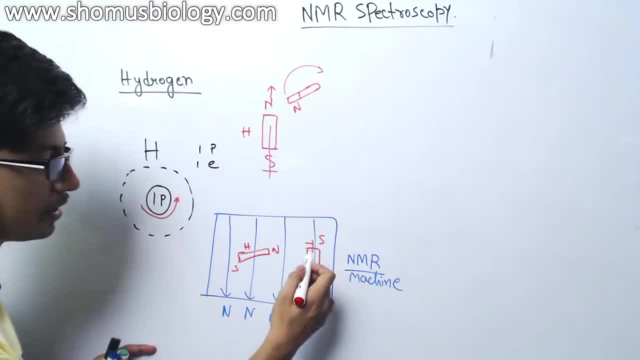 the north will be same as the north of the magnetic field, the south will be same of the south of the magnetic field. So they will be rearranged because this is the steady state, this is the most stable stable state. Okay, so let's say the normally the molecules generally. 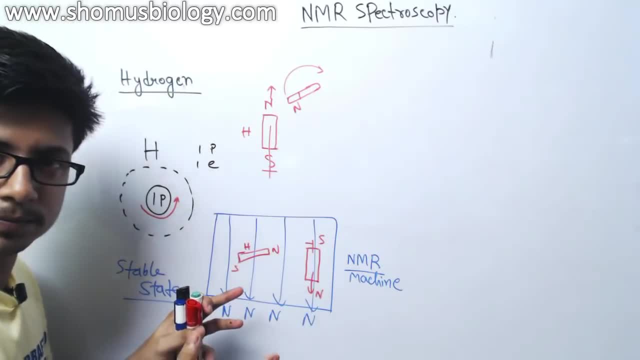 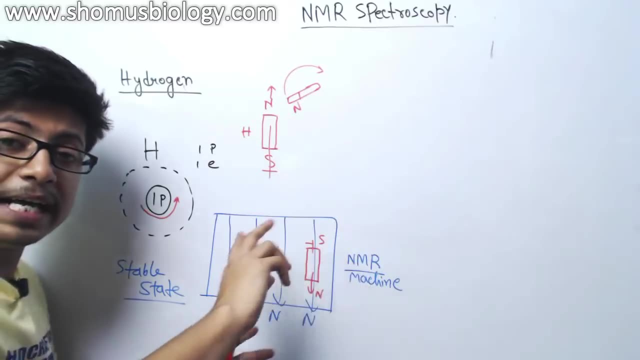 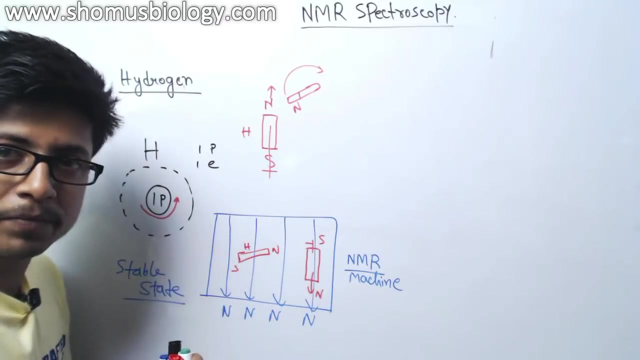 don't present like this. they present in any orientation. but the atoms present in any orientation, the hydrogen present in any orientation. but whenever we apply this magnetic field they will have a quick spin so that the match, the spin of the magnetic field, that spin is. 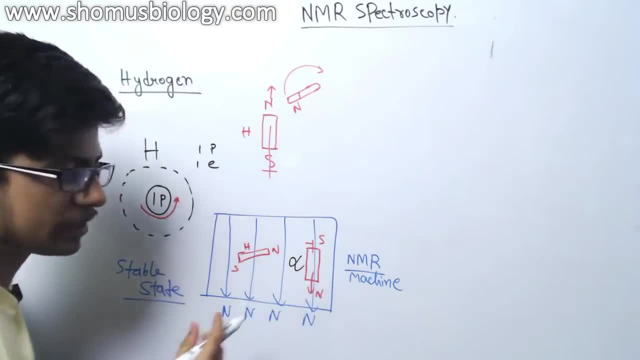 known as the alpha speed. Remember, this is known as the alpha speed. Once the speed is done, there will be rearranged to the direction of magnetic field. So this is a general idea. so what we have learnt till now? We know that 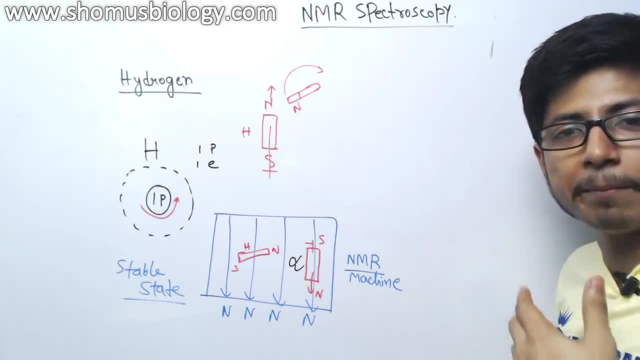 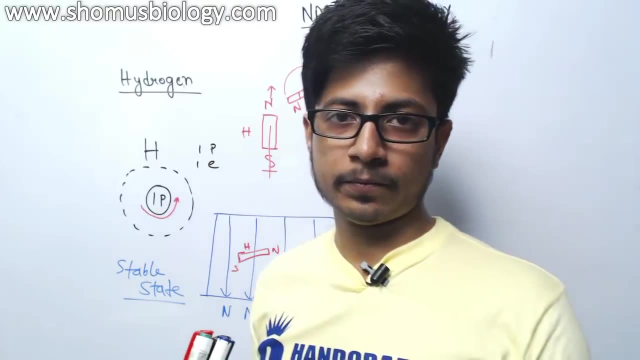 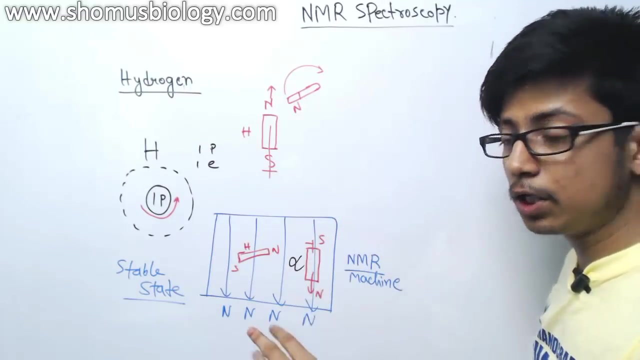 this atom hydrogen can behave like a magnet. Whenever we can apply some kind of magnetic field, it can have a spin to match that field. That's true, And in the NMR machine we do exactly that thing. We apply some magnetic field so that, according to the field, all 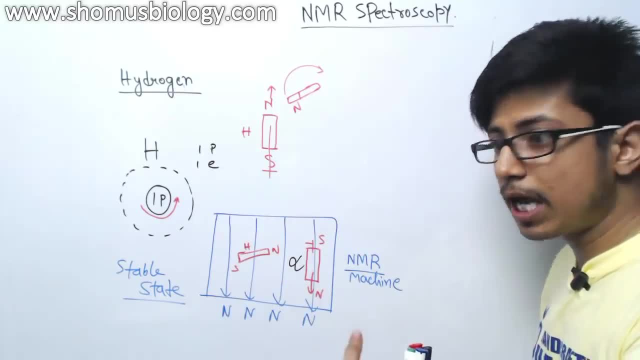 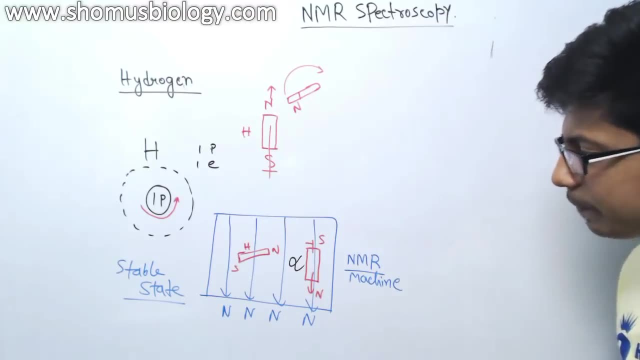 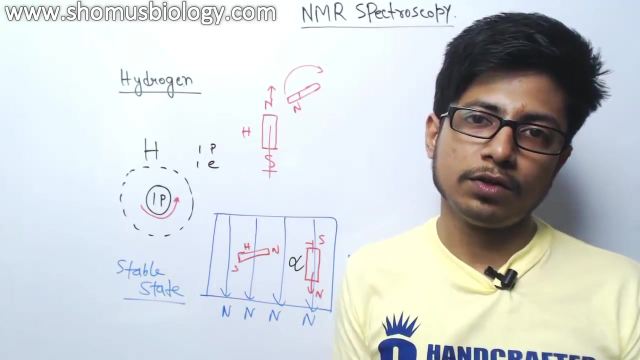 the molecules and the atoms present in the molecules rearrange according to that magnetic field. Okay, so far, so good. Now the second part of this understanding is how exactly it is going to help us understanding the structure of molecule. How do you know that? Now, this: 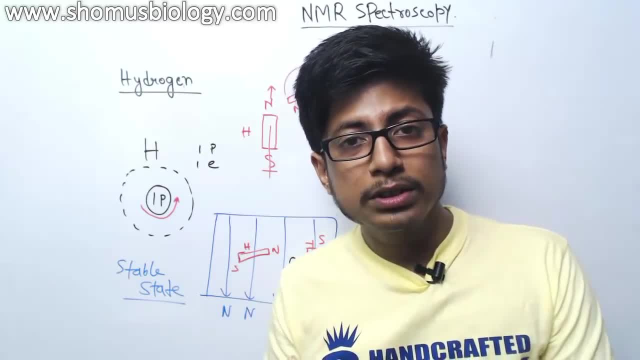 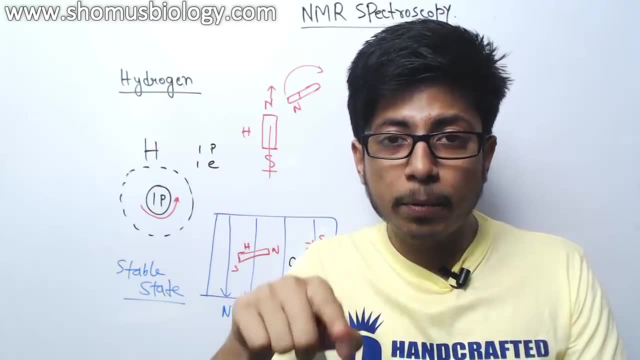 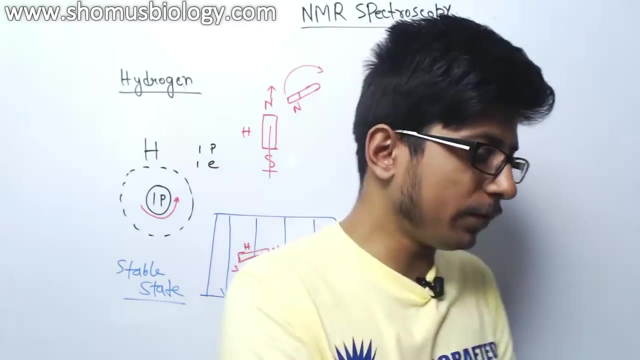 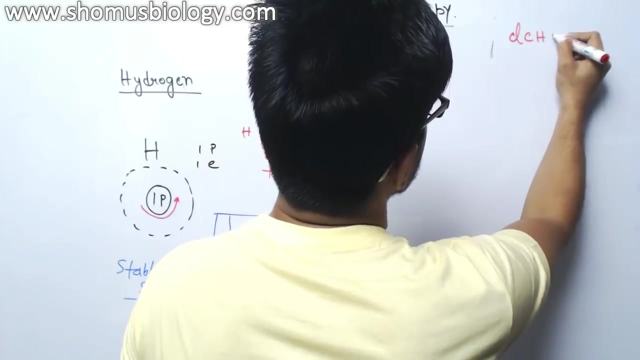 NMR spectroscopy is very important to know the presence of different groups and presence of different atoms with one another. So it's it's very important in the spatial arrangement of those atoms Okay With respect to one another. Example for that It could be chlorine, carbon hydrogen, for 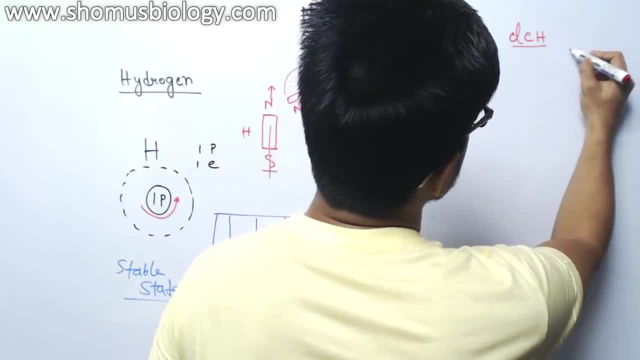 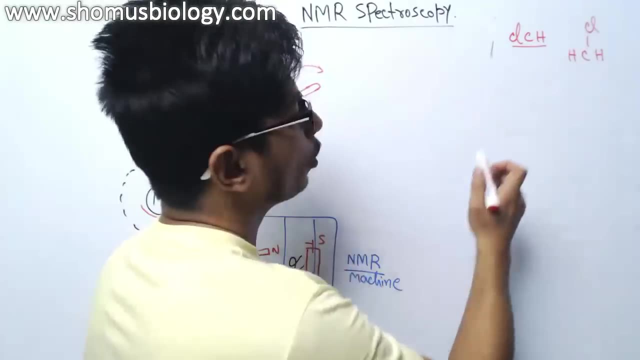 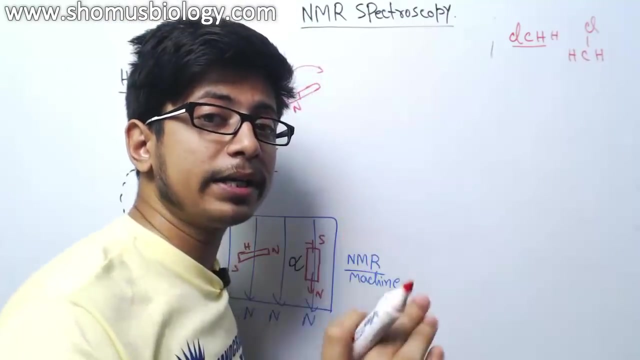 example like that. Or it could be like hydrogen, carbon hydrogen attached with chlorine, like that. So if you look at these two scenarios here, chlorine is present, one carbon to two hydrogens are present. The same thing may happen like that, but the organization and 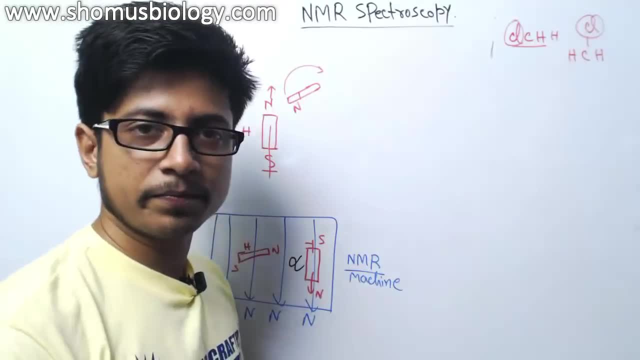 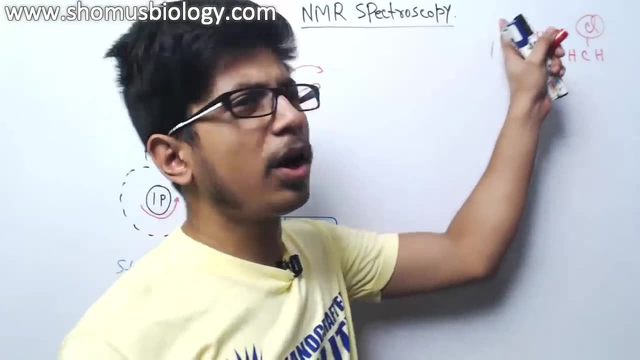 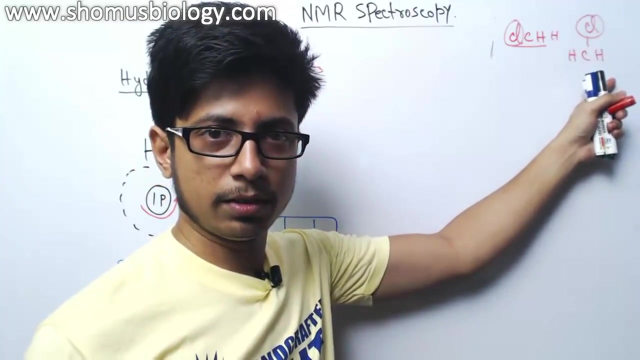 the arrangement of chlorine. Chlorine is different into these two cases, Normally IR spectroscopy or or mass spec. Those are not very good to distinguish between these two molecules because they have the same number of carbon, same number of chlorine, same number of hydrogen. So they might end up with telling: 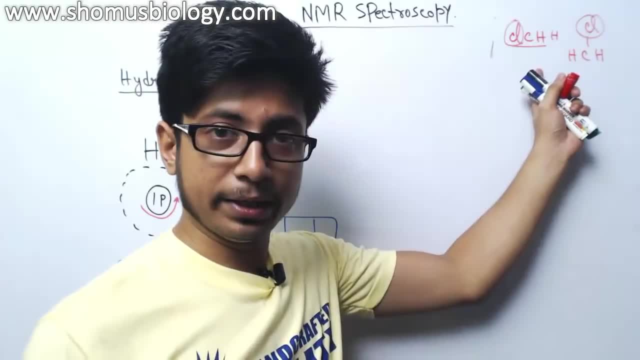 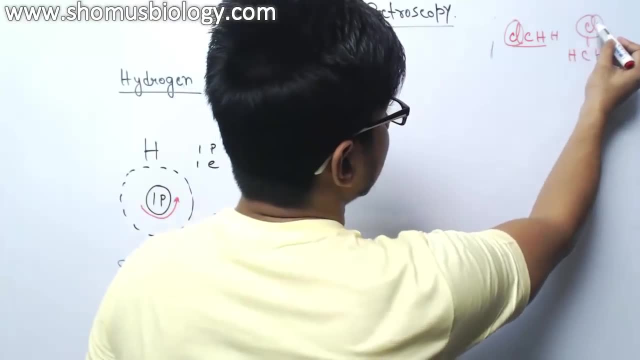 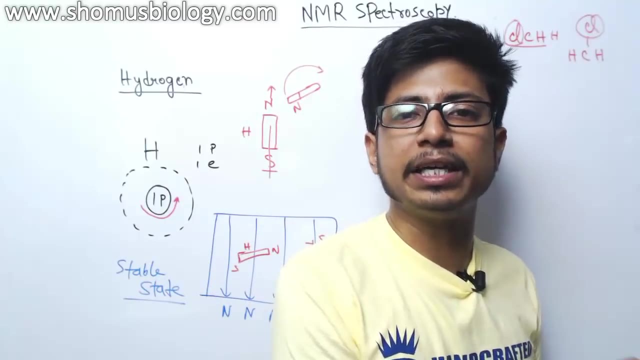 these two molecules are the same, but it can be different, And this difference can be identified only with NMR, because NMR can give you the idea about how Other Atoms are placed with respect to their positions and attachment with the nearby atom. Okay, 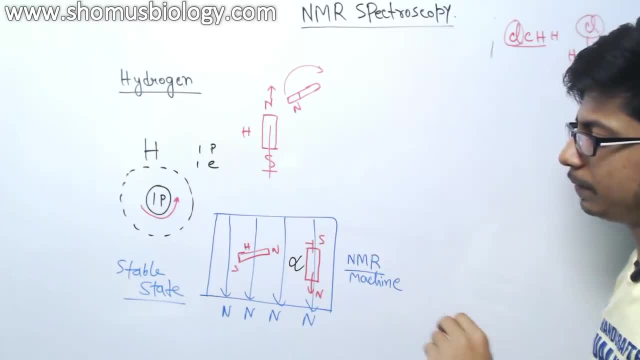 So now, if you look here, the whole idea about the spin. So we talked about till now that if you put the magnetic field, this proton have a spin, this, this hydrogen, have a spin. Now the match that, so it's called the alpha spin. So it's easy to get the alpha spin. 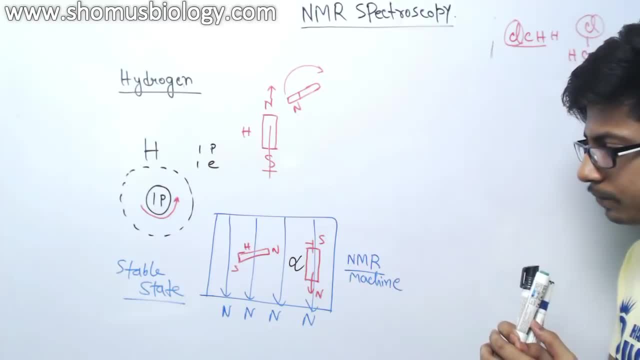 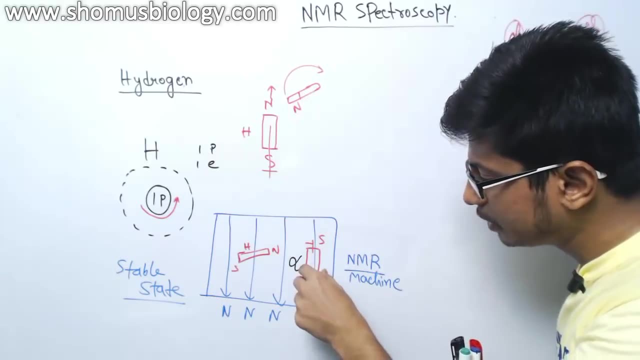 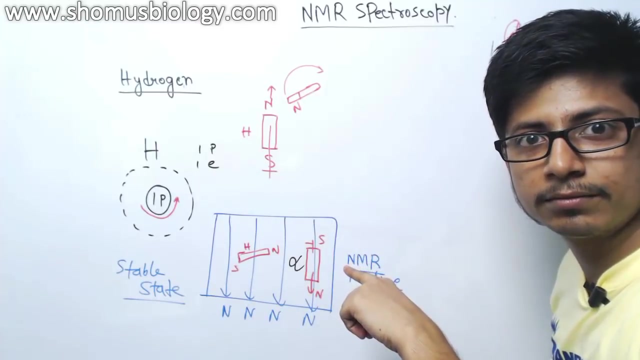 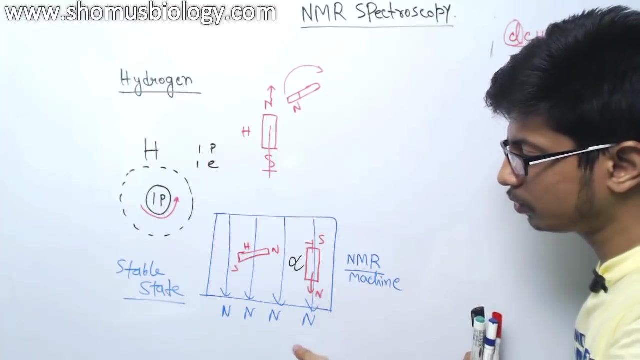 Now we take it a little far. Now what we will do now. let's say we want to apply some energy so that we can turn this hydrogen opposite direction, 180 degree opposite direction. That means we want this not to go towards the south. 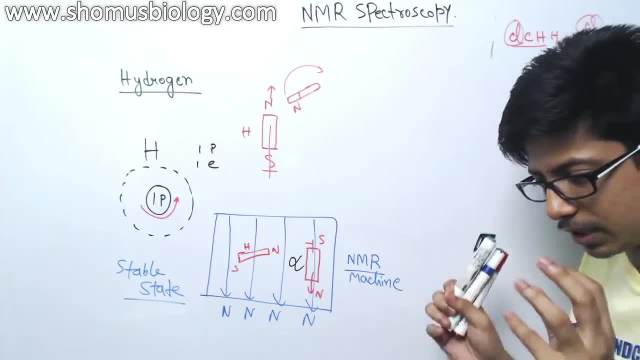 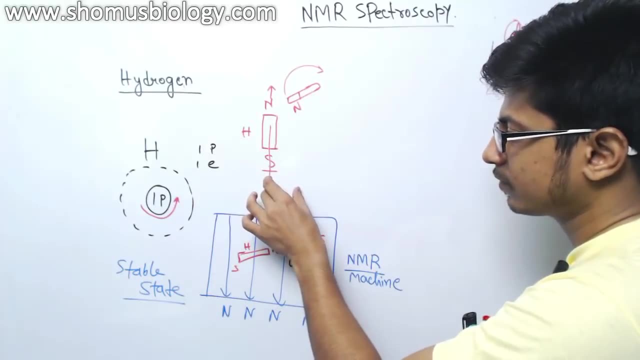 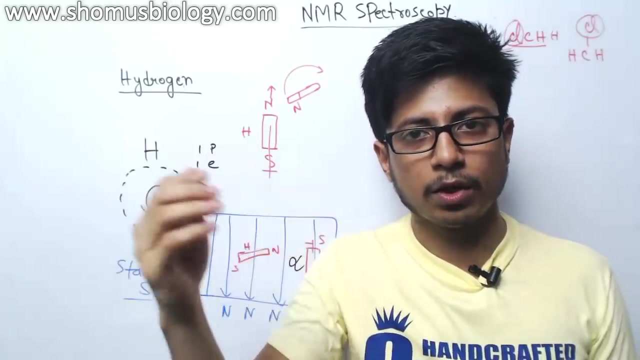 Wanted to be completely reversed, So definitely will need a lot of energy to do that. So what we do? we put a electromagnetic wave, another kind of electromagnetic wave. It's a normal light. If you look at the normal light frequency it's a normal wave. that wave or that light source can provide the sufficient. 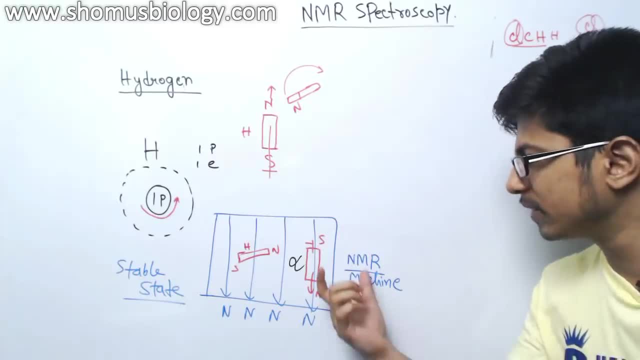 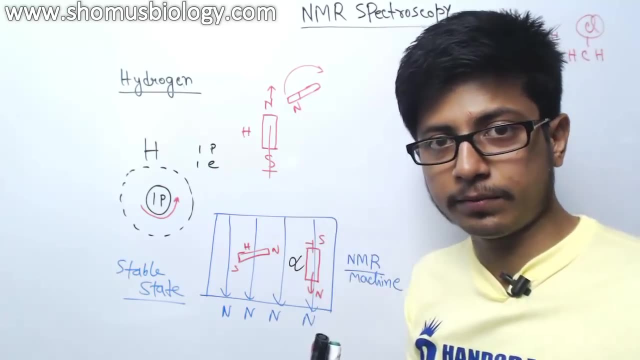 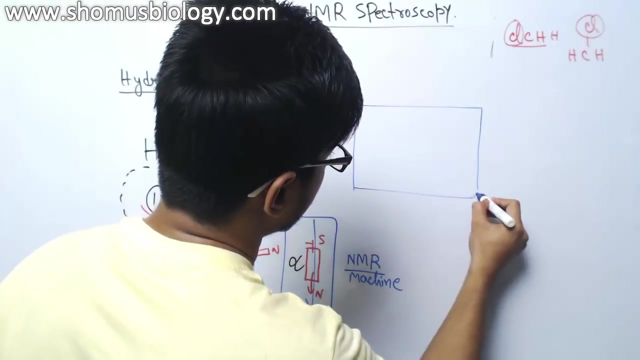 energy required for reverse spinning this hydrogen atom. So it can reverse spin when it spin back To the opposite direction. So it can reverse spin When it spin back to the opposite direction. let me draw the opposite orientation here as well. Let's say these are the directionality. 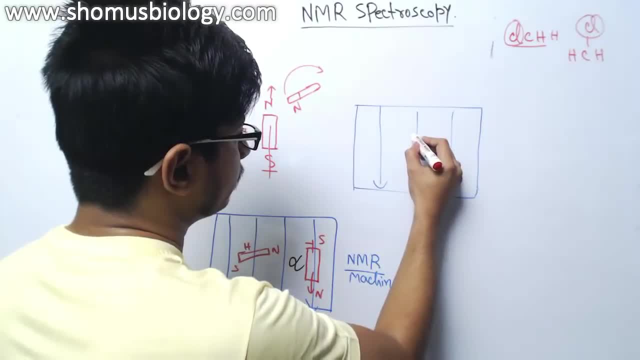 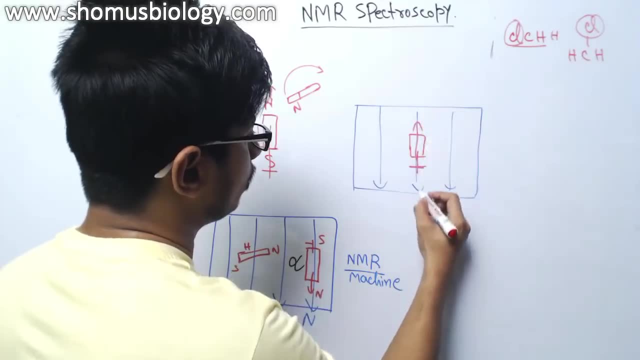 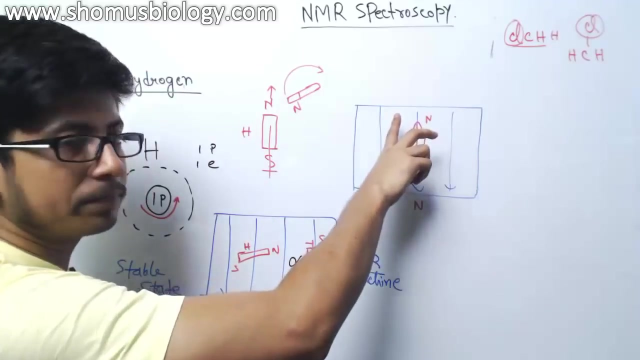 of the magnetic field, Let's say this is the one and it is organizing the opposite direction. So you see, the arrow is completely 180 degree flipped. Now this direction is completely reversed. It is a negative orientation And this is the direction of the magnetic field. 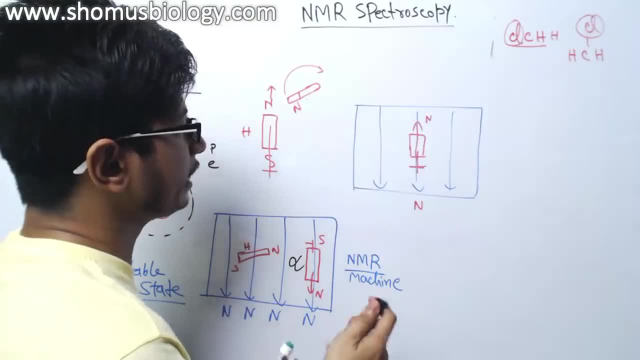 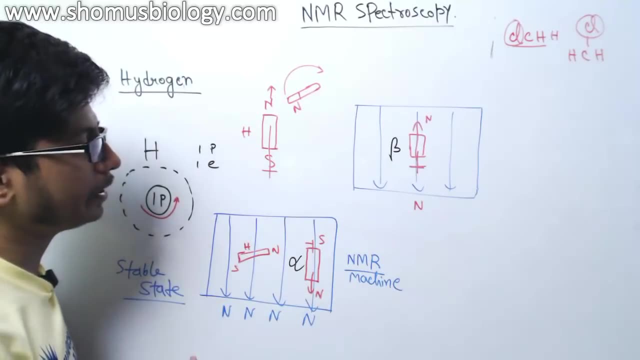 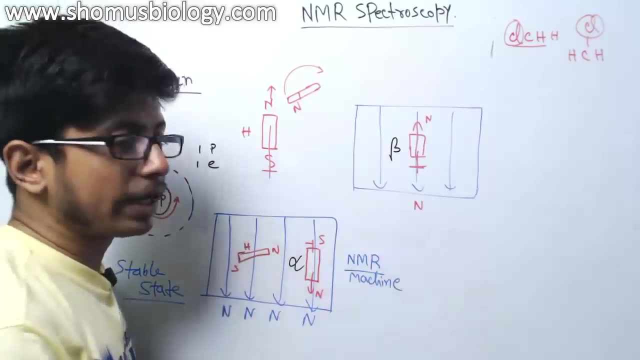 Now this pin is known as beta spin. We know alpha spin, which is the same directionality with the magnetic field, the organization, while beta spin is the opposite direction of that magnet to the magnetic field. These are the two types of spin that we know Now. 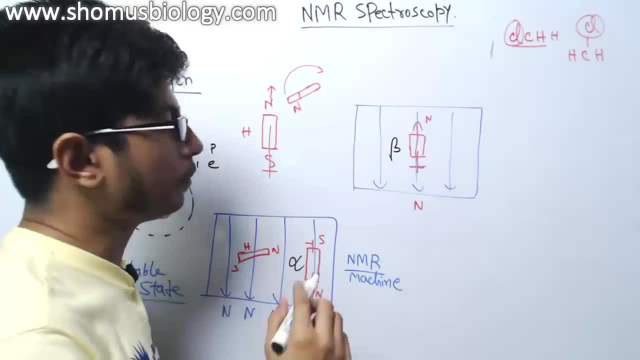 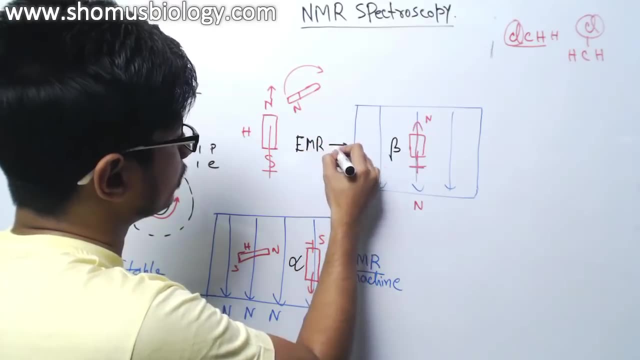 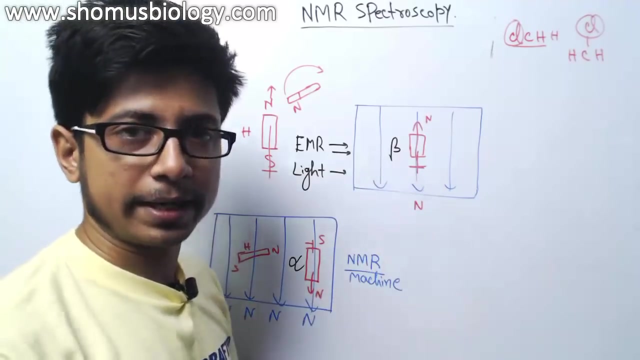 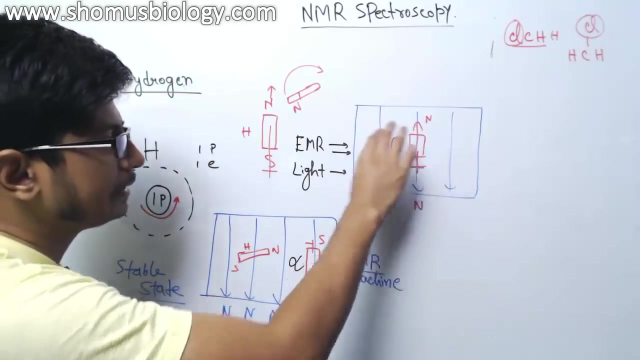 the thing is, this situation is only possible if you put some extra energy. with the help of some electromagnetic radiation, They put the wave, the light that can provide sufficient energy to do that. Okay, So once they reach this alpha to beta, we need some energy to. 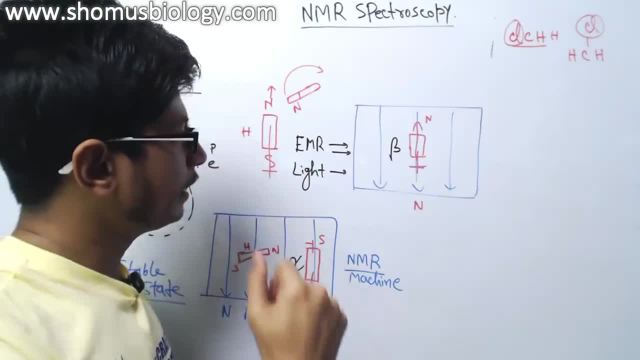 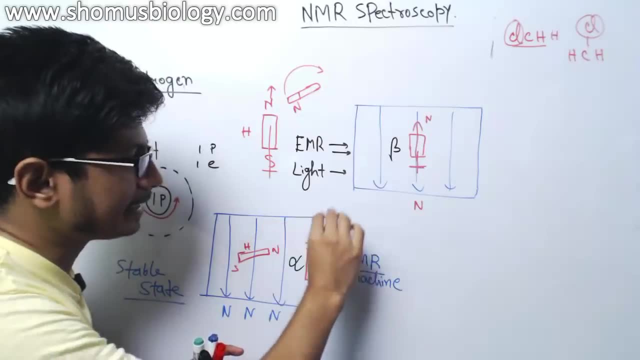 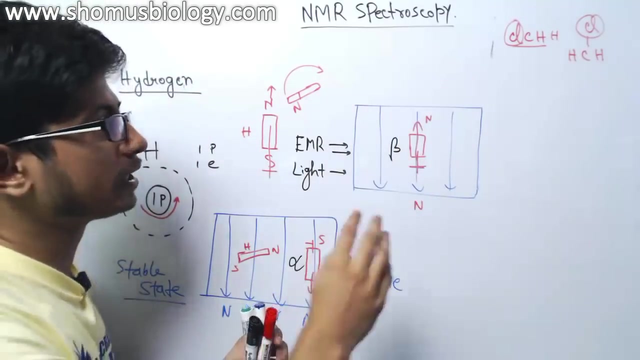 do. But now remember one thing- This is the most important point about the NMR spectroscopy, As we're talking about one type of magnet that is hydrogen, for example. Okay, Now the hydrogen, it could be different other atoms present nearby hydrogen, for example. 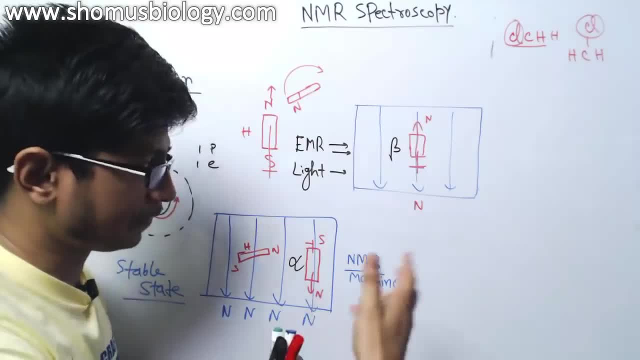 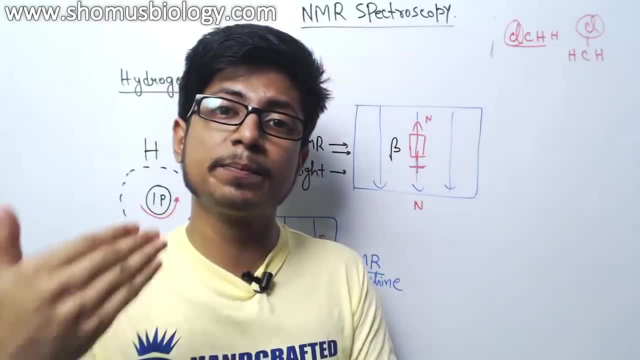 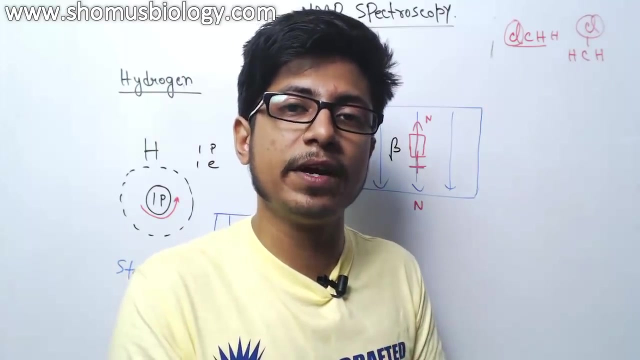 nitrogen, carbon, oxygen. different molecules can be, different atoms can be present. Now this is very important: how this hydrogen is interacting and how this hydrogen is placed near all those different atoms. That's what makes this process a technique: to specify and identify the chemical and physical properties of the molecules. For example, here you say: 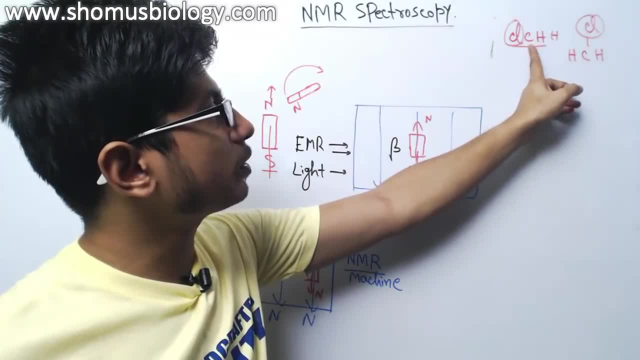 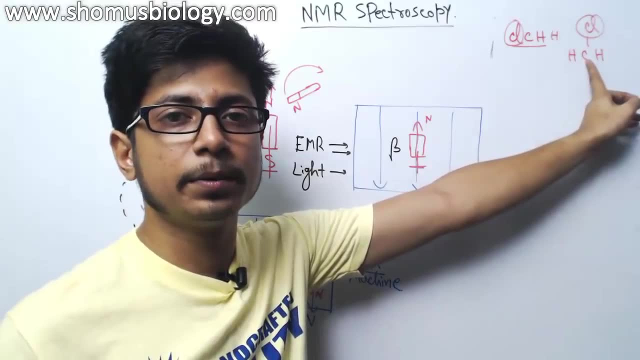 that Okay. this hydrogen is present very near to carbon here and the other one is far downside. But here you see, the hydrogen are present very close proximity to the carbon, in the same close proximity with the carbon. so depends how exactly hydrogen is arranged. that is the 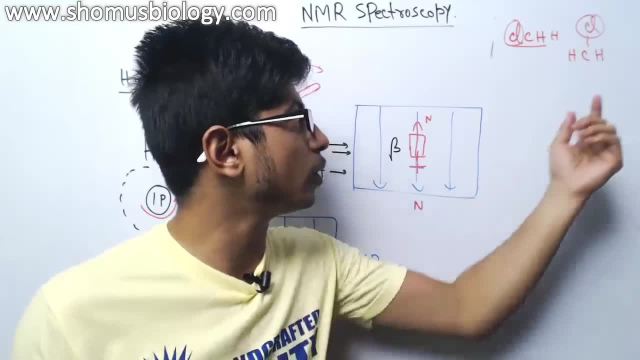 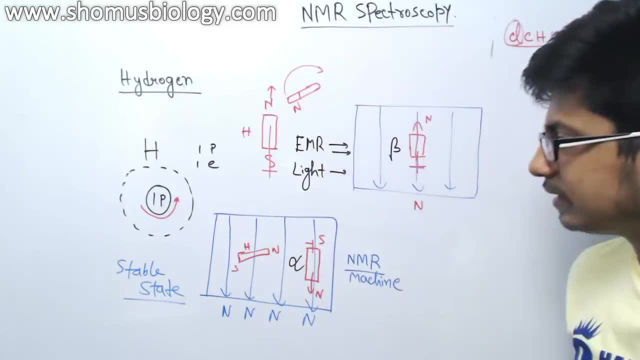 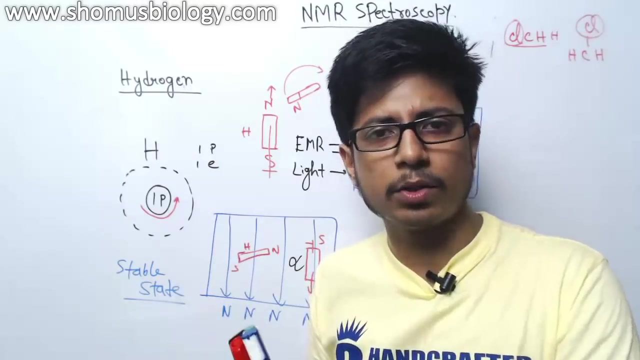 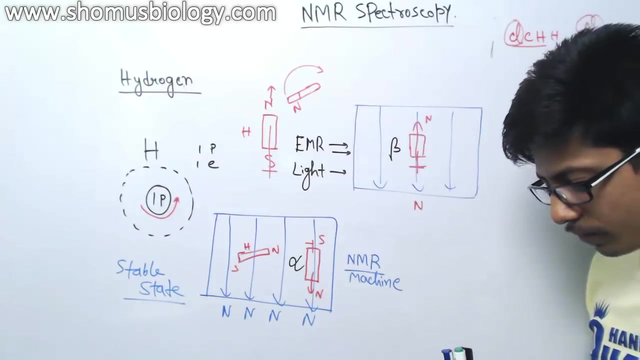 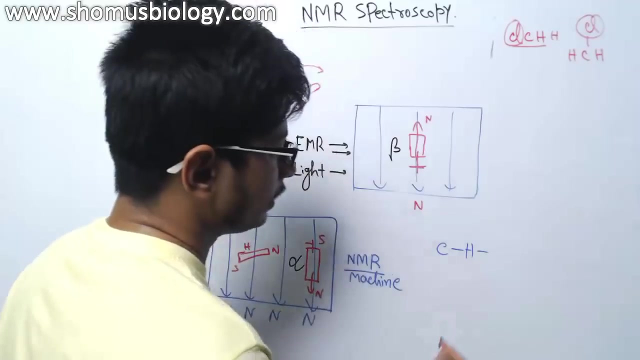 proton are working as a proton Here. all your the presence of other molecules near hydrogen, other atoms- and very sorry, it's not molecule- other atoms near hydrogen changes its behavior. Let's look at that Now. let's say, let's say, hydrogen is present. Carbon is also surrounding that hydrogen. What does that mean? Hydrogen? 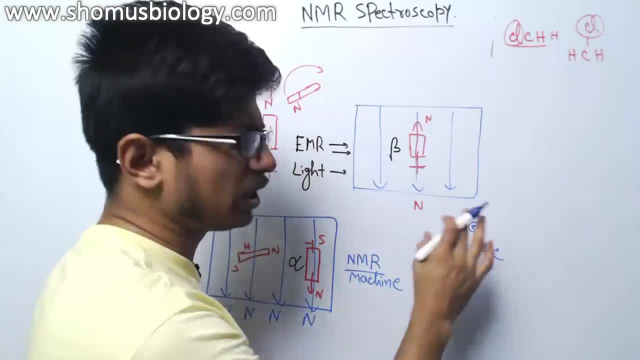 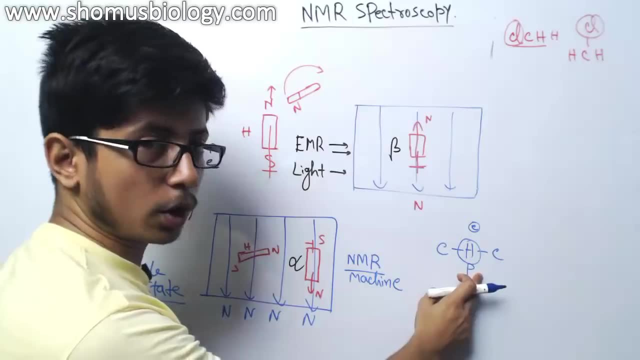 have only one electron and we are not going to talk about that much because it's only one electron. The effect is not that high, but it has the proton, only one single proton. and we're talking about the proton because it is the protons feature to give us the magnetic. 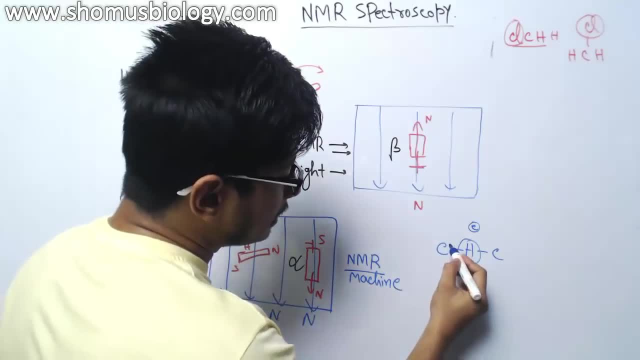 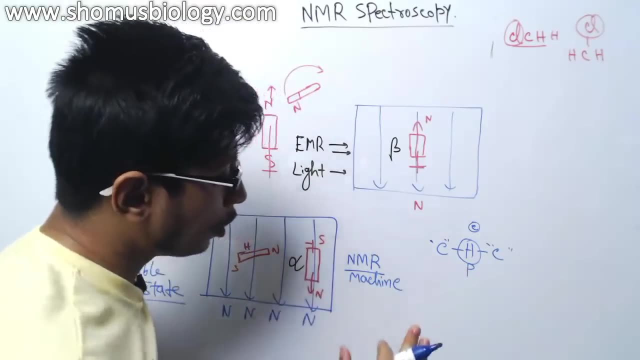 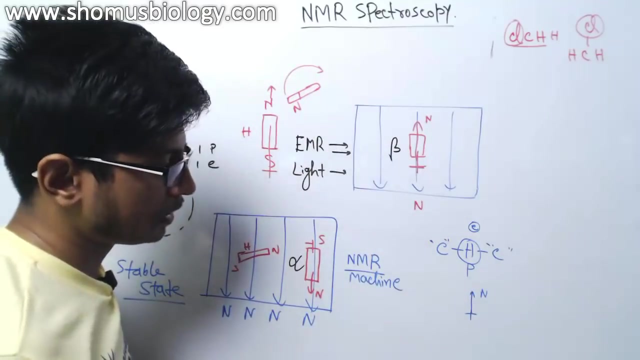 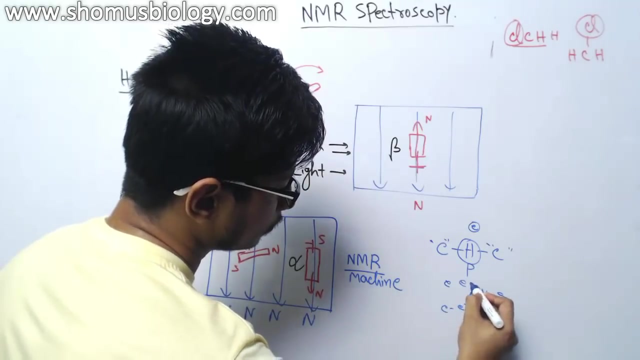 field or give a behave like a magnet. Now, this nearby carbon molecules contains a lot of electron. right, They contains a lot of electron. So the idea is this: protons sometime. that said, this is the proton acting as a magnet. This proton is surrounded by a lot of electrons, So this magnet is masked by a lot of electrons. We 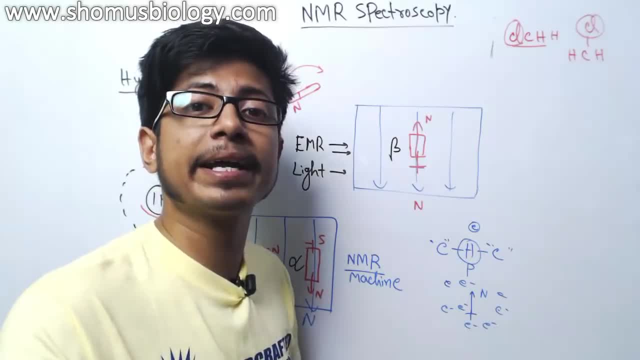 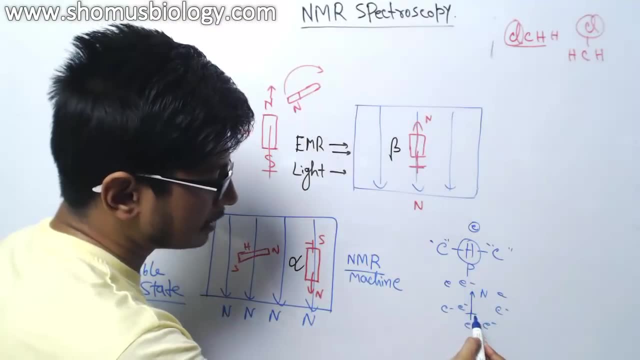 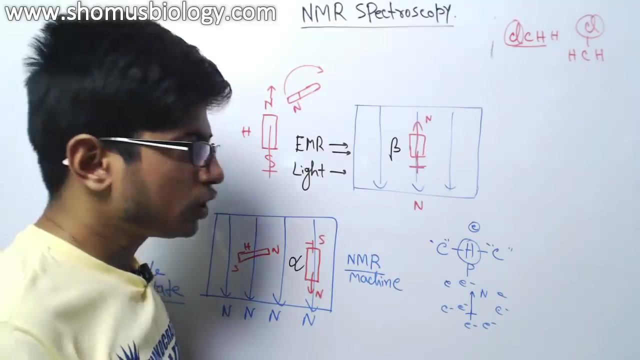 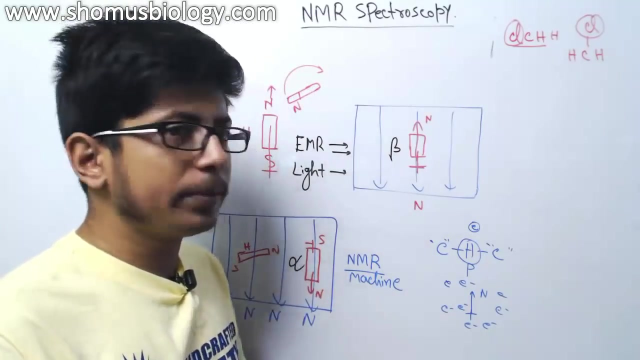 call it as a magnetic shielding or call it a die magnetic shielding. This die magnetic shielding is actually preventing this magnet feature of the hydrogen. Okay, so for different molecules this magnetic shielding could be different, right? So let's take a molecule where we have. 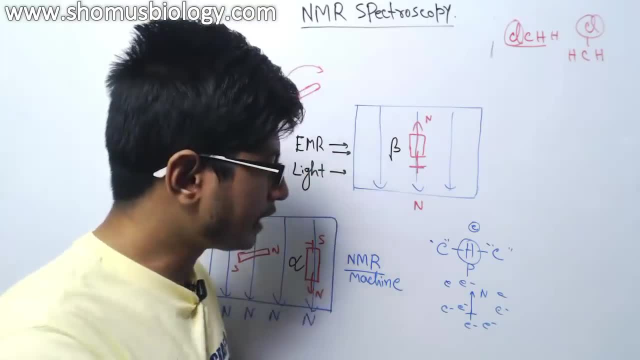 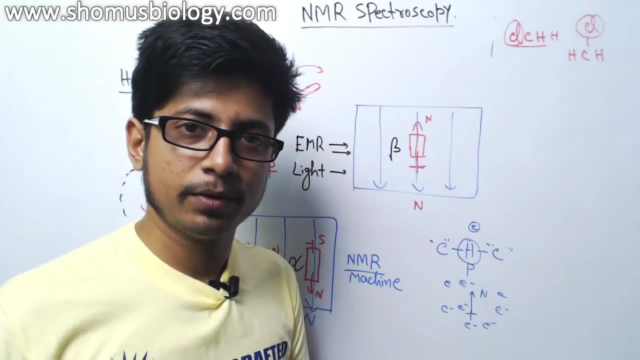 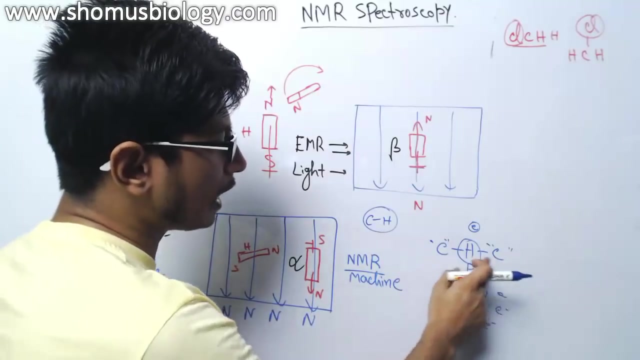 only one, hydrogen, and let's take another molecule where we have hydrogen attached with carbon, two different carbons, for example nearby right. Or let's say, take one molecule where we have one carbon and hydrogen and another molecule where you have two carbons attached. 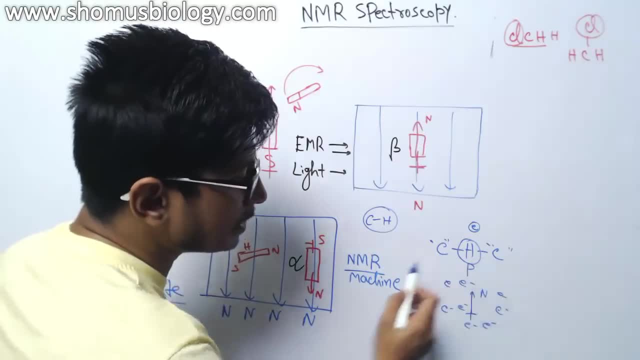 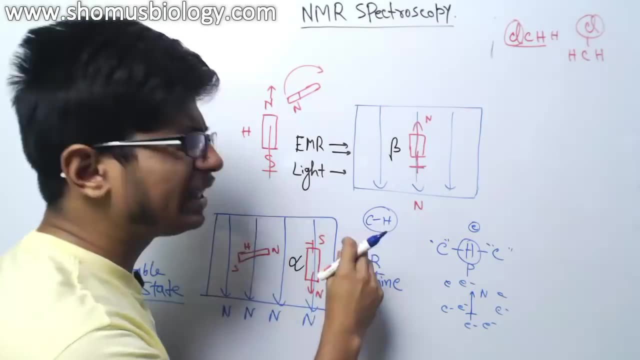 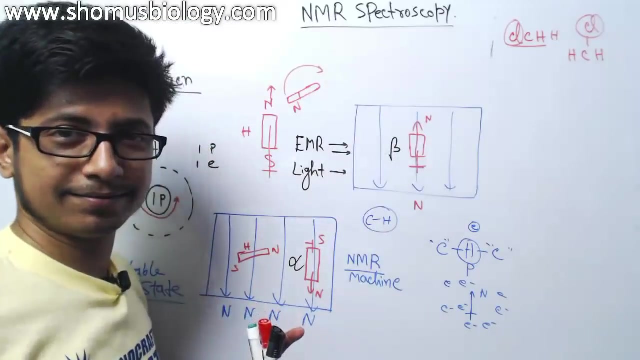 to the same hydrogen. So as there are two carbons present, this second one will be more shielded. The first one have only one carbon, so it will be less shielded. So what does the shielding affect? the whole idea about spinning. Let's look at it. The idea about 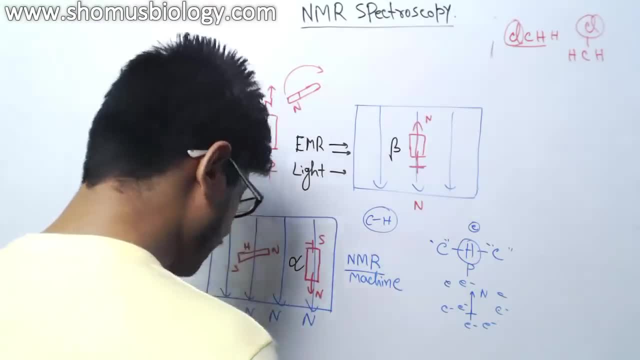 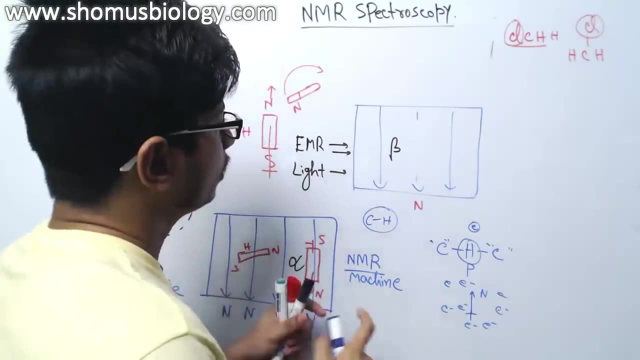 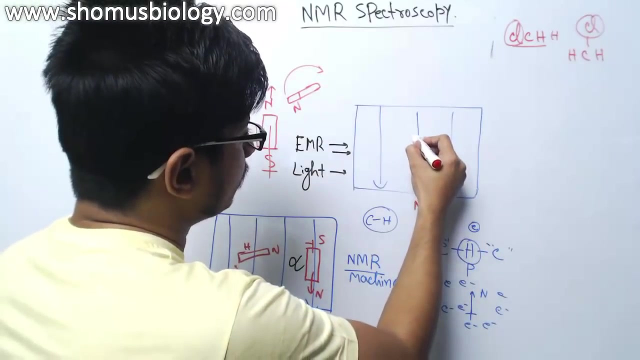 the spinning and shielding. again, I have to. I have to draw that. this is the same scenario that we are talking about. This is the direction of the magnetic field in the NMR machine and- and this is our proton- This is a hydrogen that we're talking about. it is in the alpha. 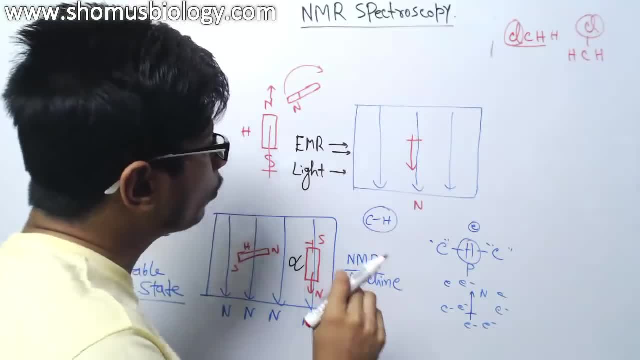 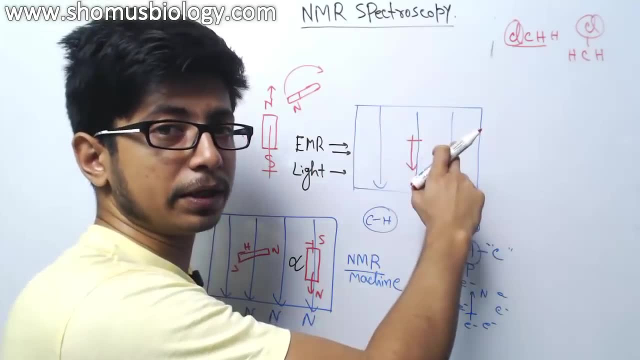 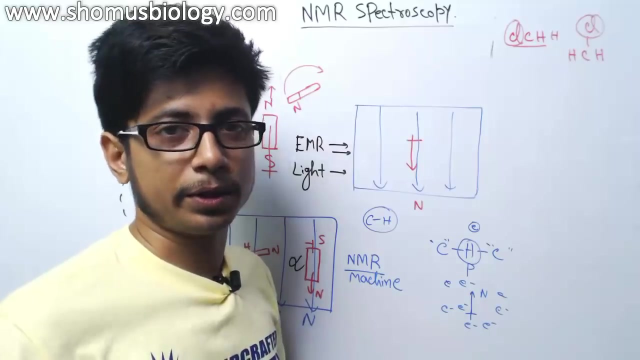 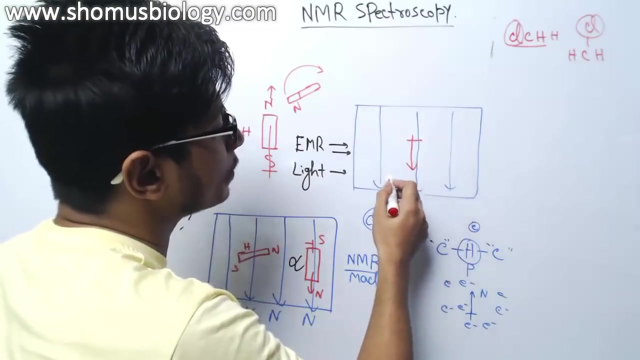 spin mode. Now I told you that we want some time this, this magnet, this hydrogen, to be completely reversed, spin to the beta state. So this reversing is will be different for different type of molecules, depending upon the presence of those electrons. If there are no electrons present surrounding this hydrogen, the magnetic effect will be very 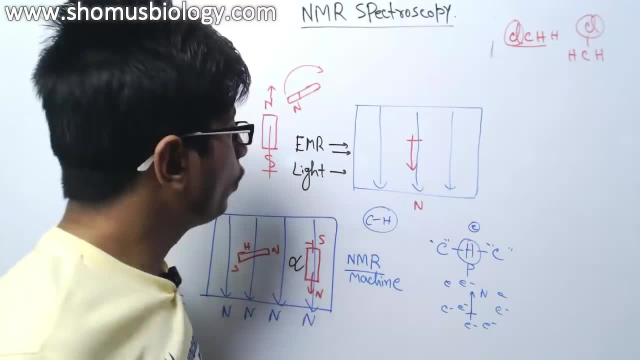 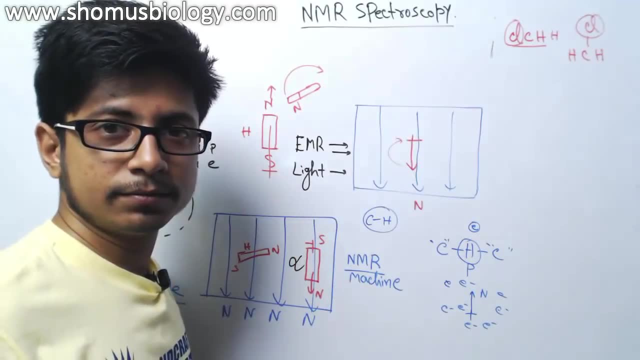 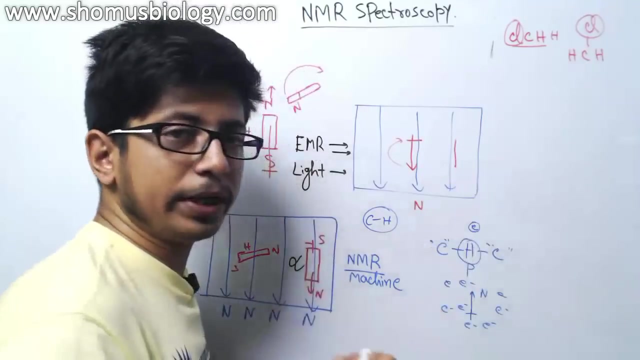 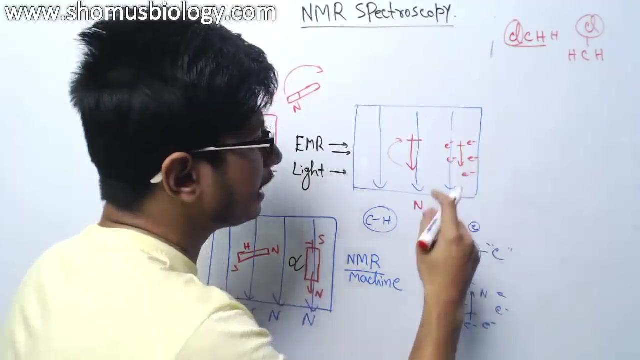 high in that sense. So what we need? we need more of this energy, more of this energy to shift it to the beta state. Okay, but let's say, if this same scenario- and it is filled with it- is filled with electrons, surrounding with electrons, These electrons, 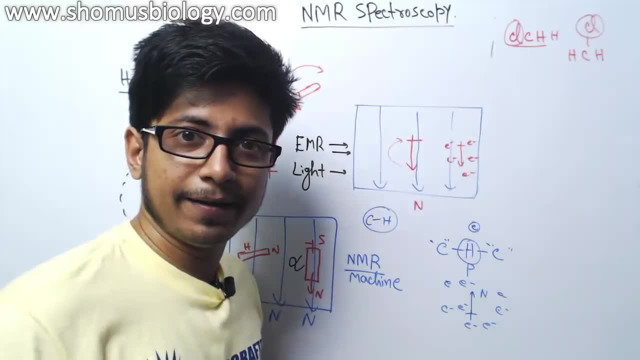 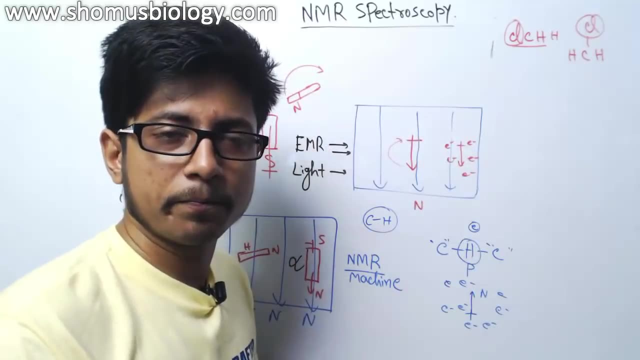 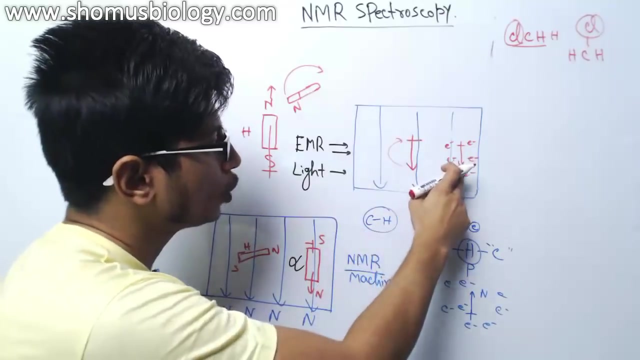 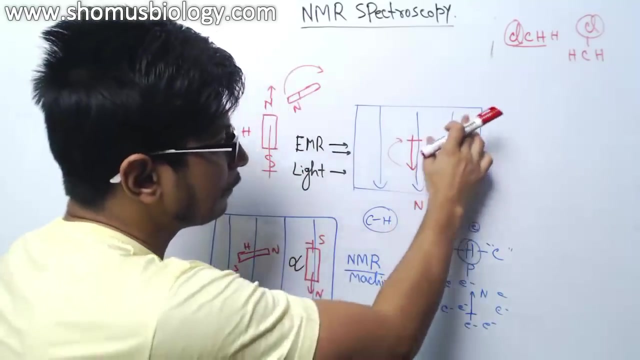 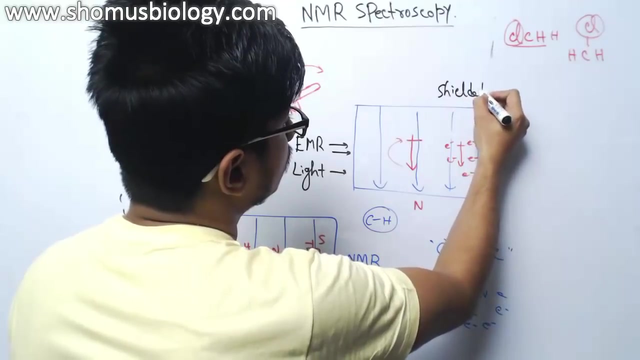 are masking the effect of the magnetic field. So the effect of magnetic field is not that high in this hydrogen atom. So we need less energy as electromagnetic radiation, electromagnetic wave, to put it to the beta state or beta spin state. Got the idea. So if if it is shielded, we need less energy to spin it back to the beta. 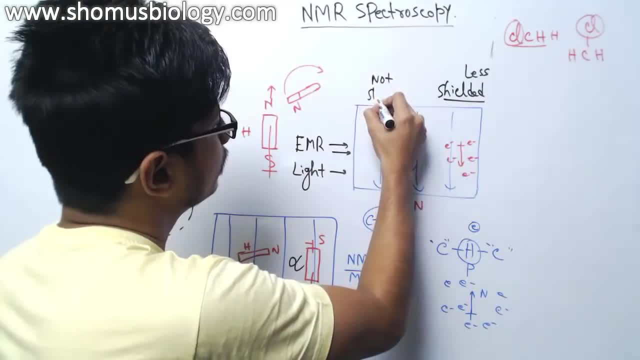 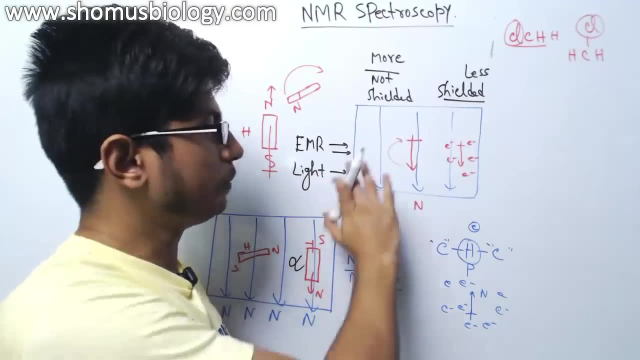 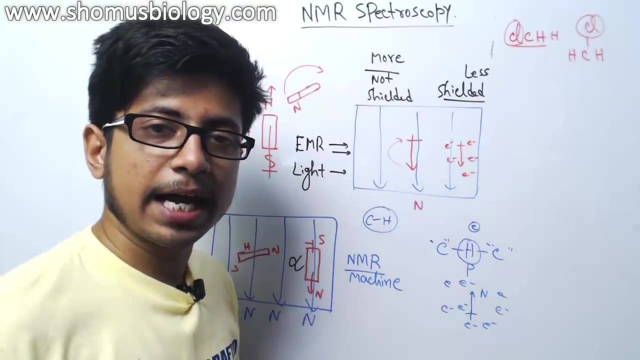 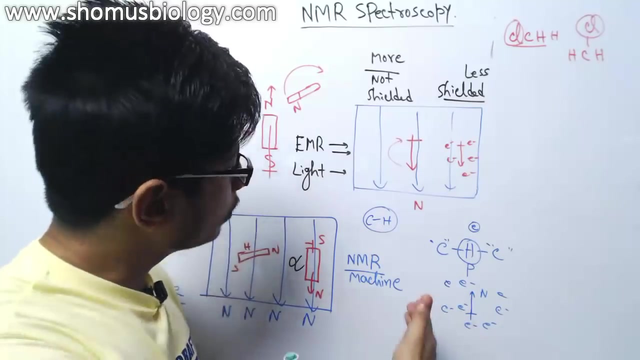 state. If it is not shielded, we need more energy to put it back to the beta spin state. This is the most important point that helps us to find out the structure and the arrangement of different protons and different atoms in the molecule. Okay, how let's look at it? This is filled, So I have to erase this, and 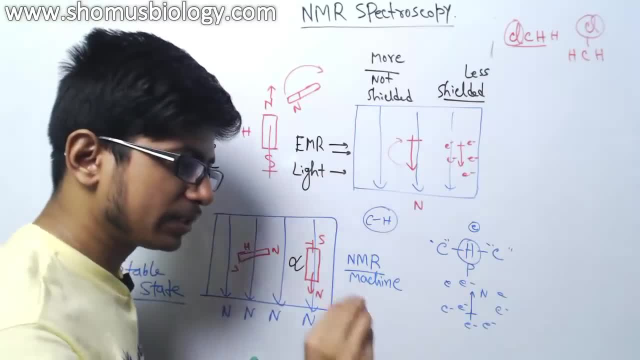 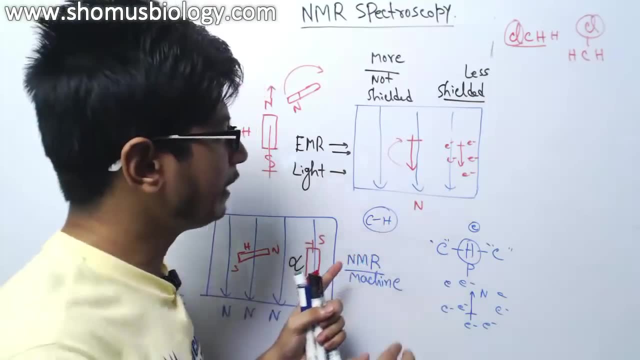 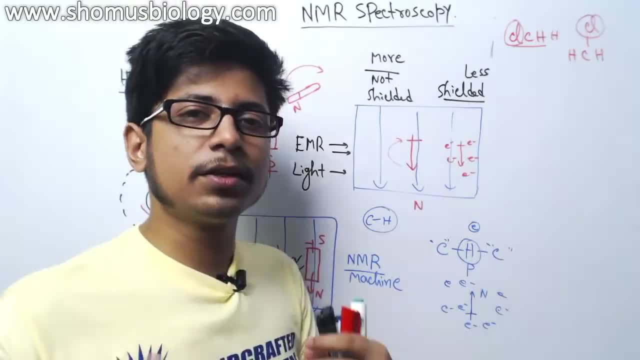 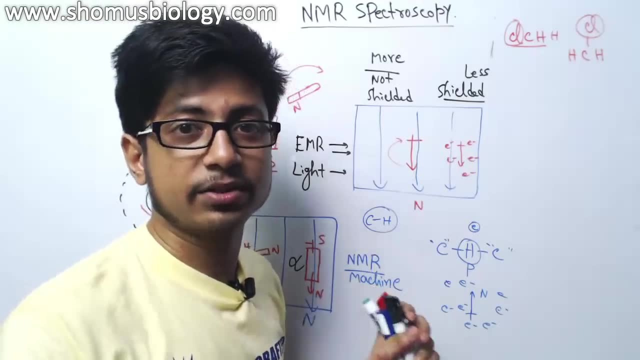 let's say. let's say, this battery is issuing different bonding of these atoms And, due to the presence of different atoms nearby, the shielding annunciating will take place and that will help us to find out the exact structure. Okay, so let's look. 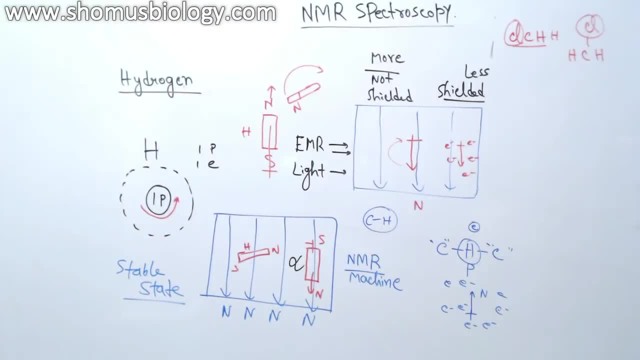 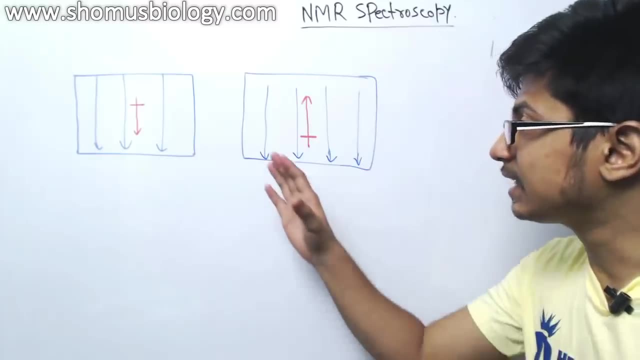 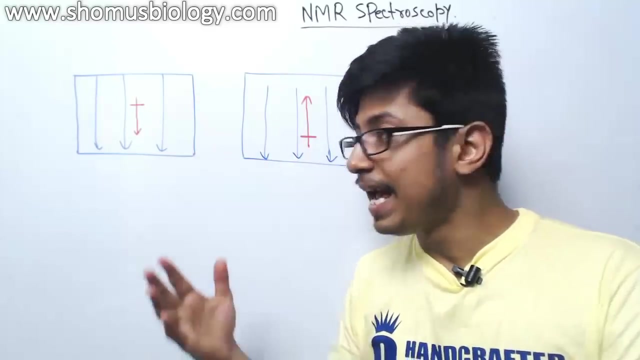 at that in a moment Was good, The one that is, this idea of spinning the magnet back 180 degree to the beta spin state, and so this it, And that thing is known as the resonance. Resonance Why? Because, if you're talking about 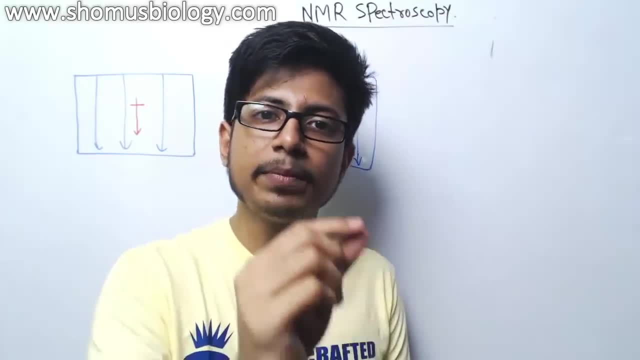 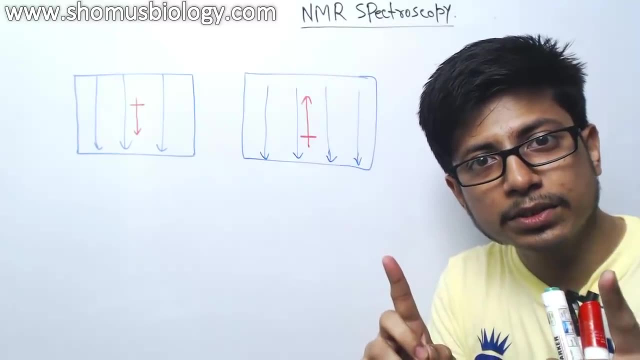 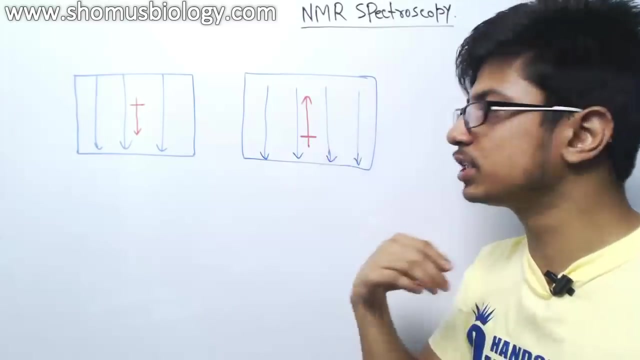 consecutive atoms that are linked with a single, single atom. if we're talking about that, resonance means we want to put all those atoms, or all those hydrogens that we're dealing with, which are behaving like a magnet, to the same orientation with the magnetic field. that will be the opposite. 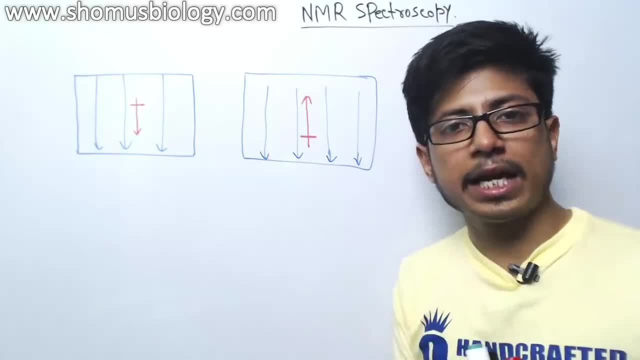 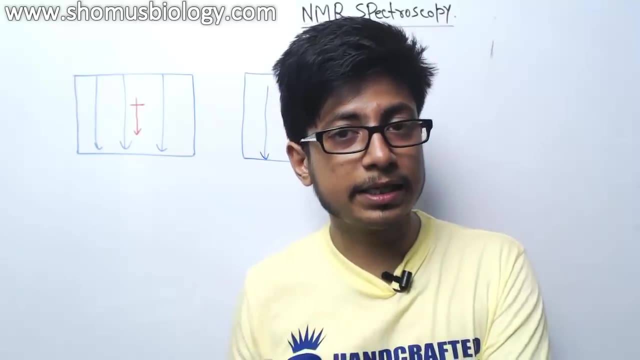 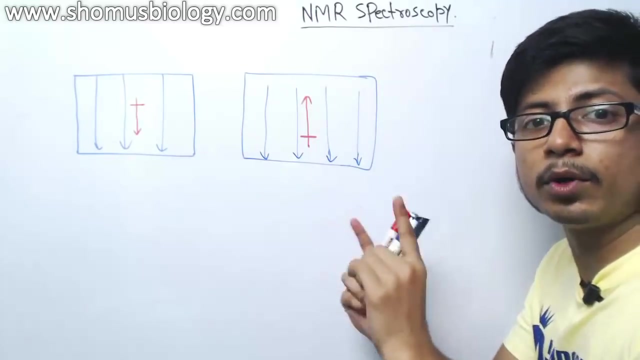 of that magnetic field. Okay, so at a time, if you're dealing with a molecule structure, we will, we will. we definitely want all the hydrogen that is present in that atom, that is present in that molecule that should be spinned in the same direction, same orientation. 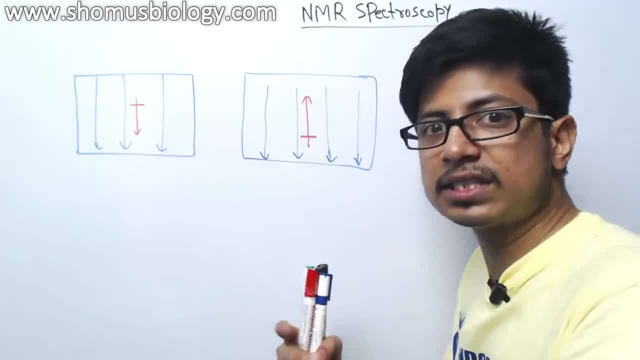 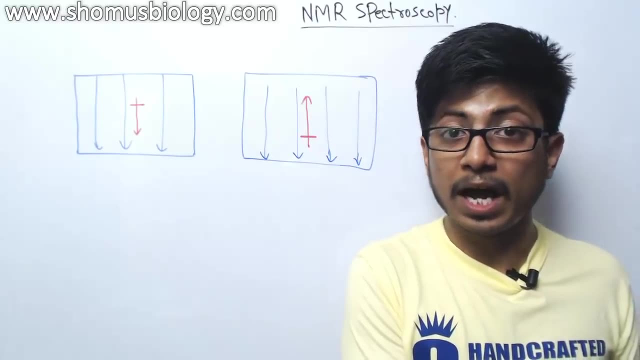 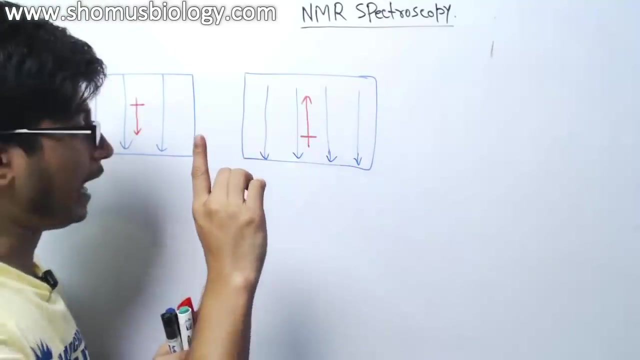 and that same orientation of the spin is going to give us a data that is going to help us to understand about the structure of that molecule. How? because, as we are telling all those hydrogen to get a same type of arrangement, which is against the magnetic field, this is known as a resonance, because resonance means all. 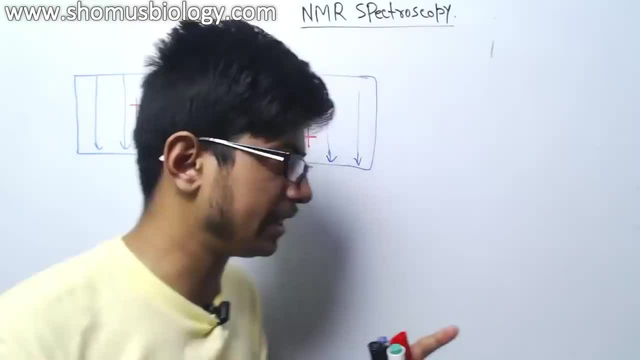 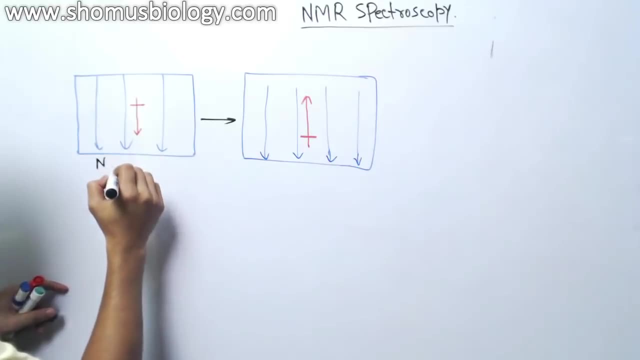 those other atoms are doing the same thing at the same time. that is called the resonance here. So the idea is very simple. Earlier the hydrogen was present according to the magnetic field, the direction to the magnetic field. Now we apply some energy here, the 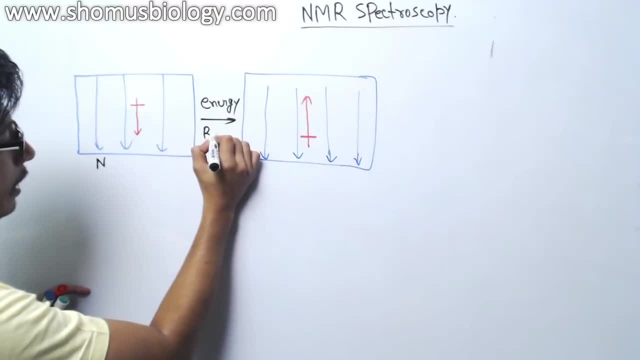 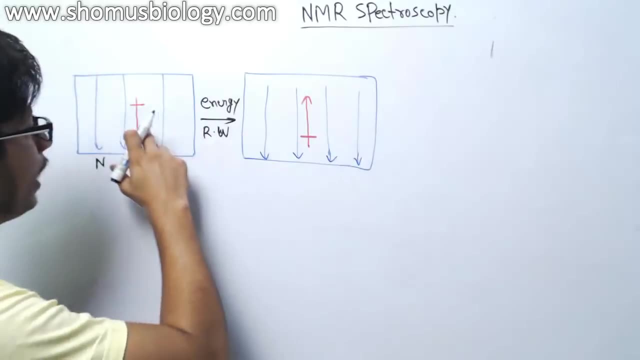 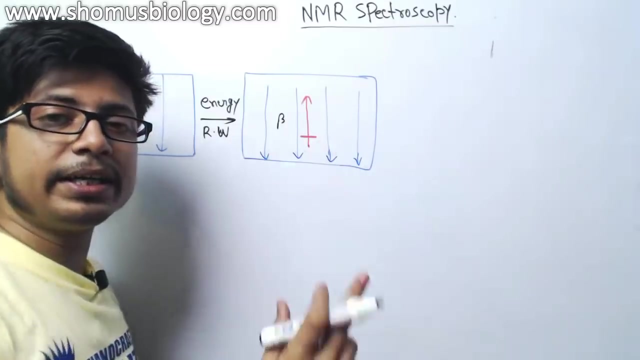 energy is applied with the radio. So the deceived they kalau electromagnetic wave or radio vitekan you can. you can tell that in shift this orientation of this hydrogen to the opposite sides. to be of a bit, us been here Now for a orienting into the beta spin. 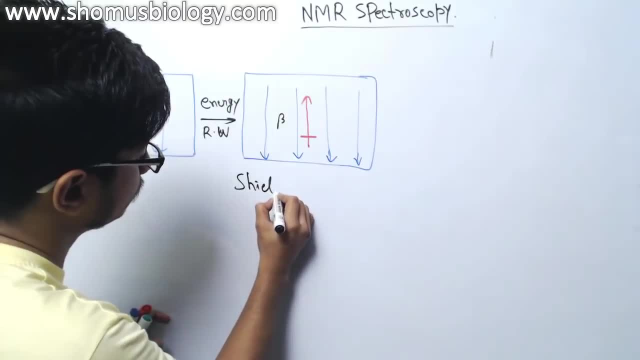 as we saw, if it is shielded by electrons, we need less energy. So if it shielded, less energy. if we are aeletrons, we need less energy if it is de shielded By electrons. So if it is shielded, we need less energy. So if it is shielded, Let me plant like this, this here, let me share Rederd운 cima r occupation That, if we look at the reference, we already have ten times this cleans source, etc. in spectrograph union takeaway. but whether there is an effect which we already masks, We will. 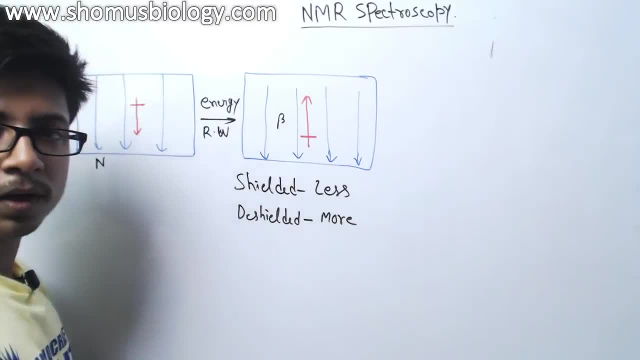 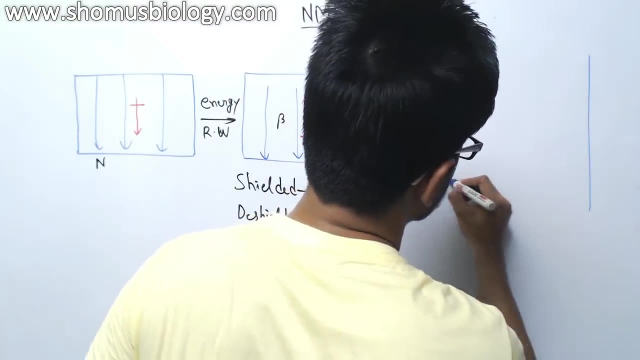 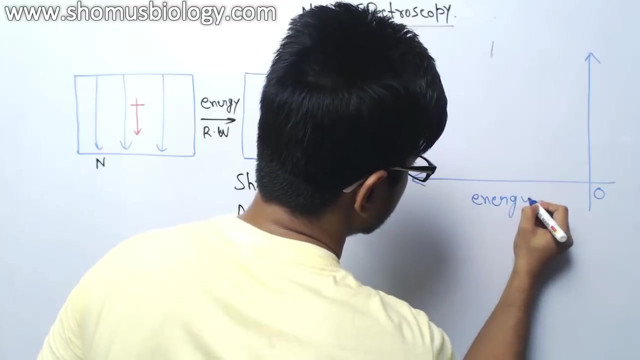 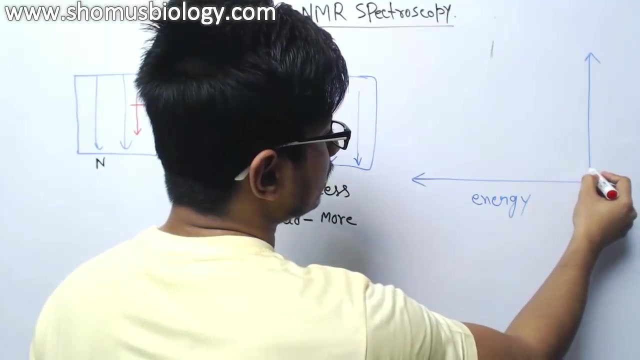 we need more energy. So what we do, if we do the graph, let me, let me do a structure or a graph. If we do a graph in the x axis, we have the energy. Okay, so what we will find here is that they will be like like at the. from the beginning, there will be peak. 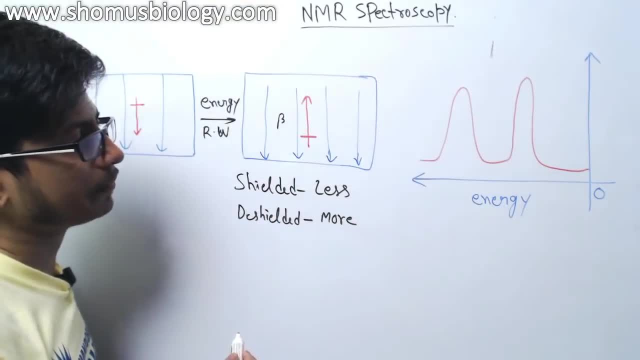 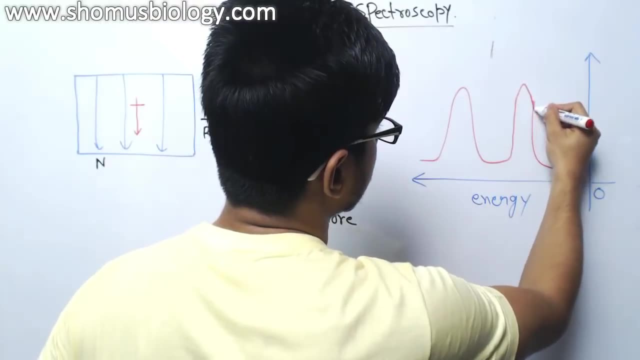 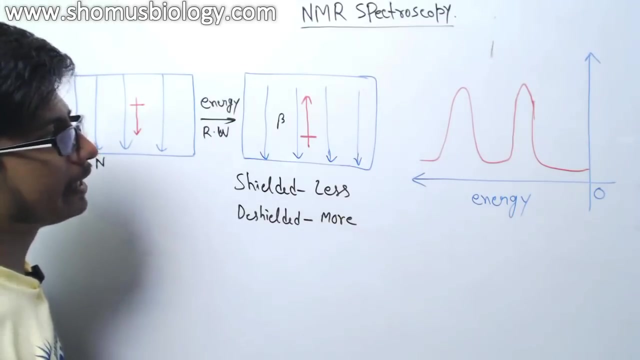 that we observe, peak that we can see, based on the same hydrogen that we're dealing with, length will be the same as the height, in the sense not that blunt it is okay. so this kind of peak that we'll observe Now, for example, say there is a shielded and deshielded two. 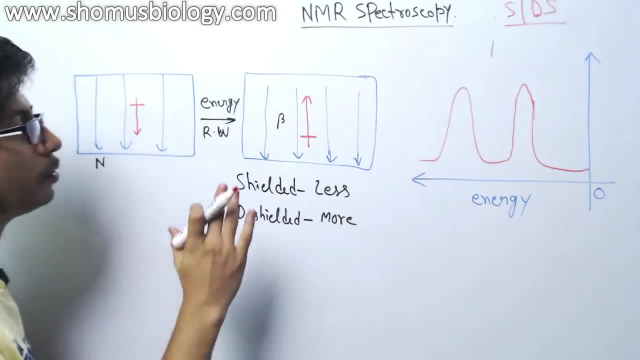 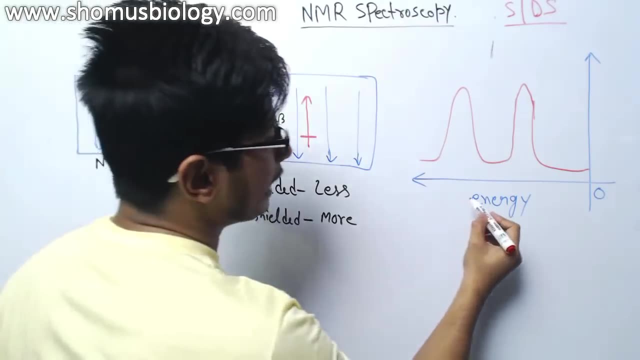 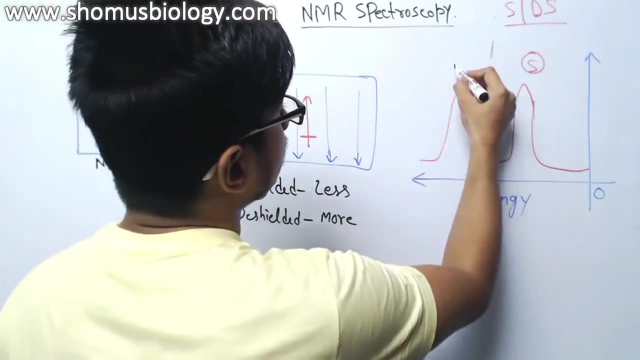 types of magnetic situation. we're talking about two types of hydrogen. we're talking about for the shielded one. Remember, we need less energy, So the energy that we for the shielded, which will be less, which will be deshielded, that will be here. Okay, shielded and deshielded, We have this. 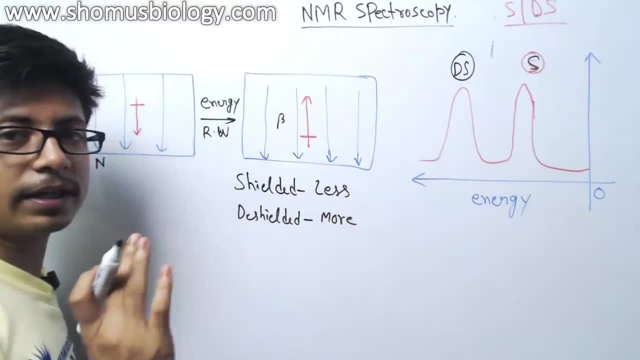 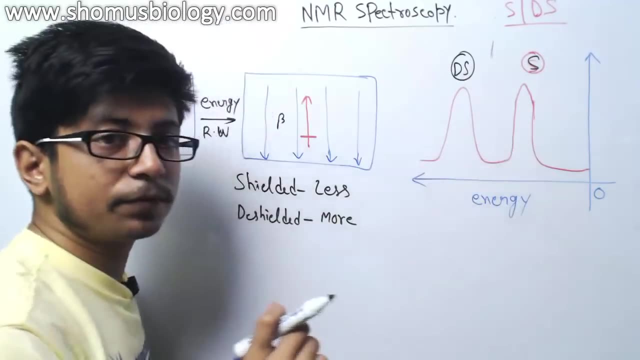 kind of graph for that. So this kind of graph is going to tell us about how exactly it is organized and how exactly we're talking about Now think about the same graph if we're dealing with a molecule which which have multiple hydrogens attached with different types of. 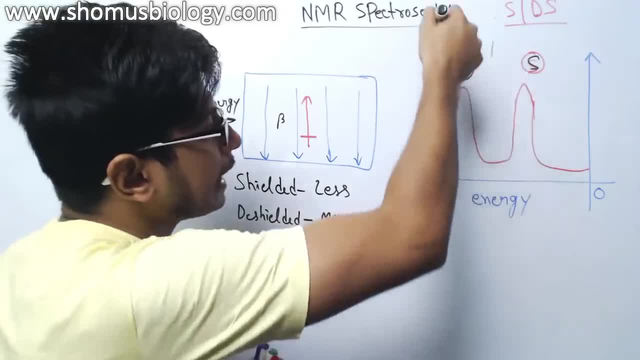 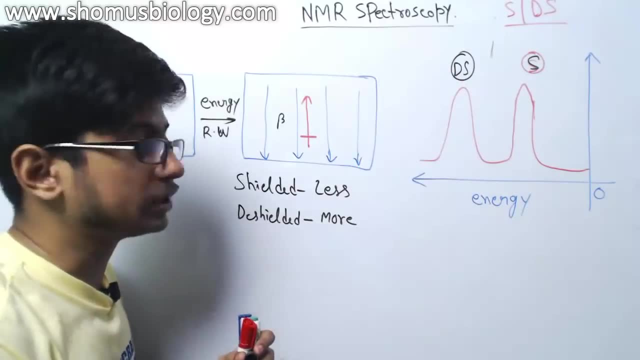 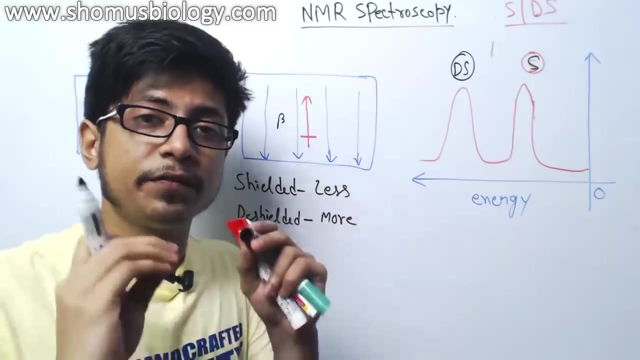 different molecules there at a different atoms. we have a different kind of graph and the pattern of the graph is going to tell us about what kind of atoms are organized and arranged with each other, where exactly the hydrogen is present, how many hydrogen is present or not, Because here hydrogen is very important and the presence of hydrogen 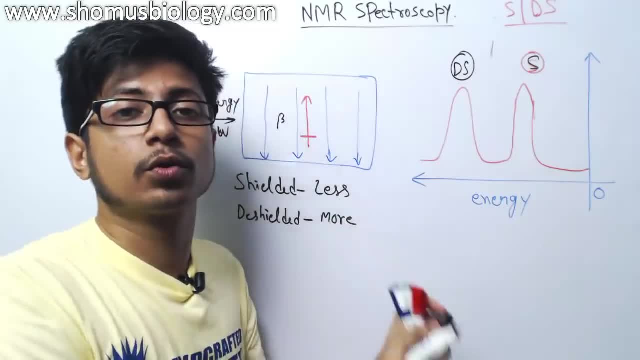 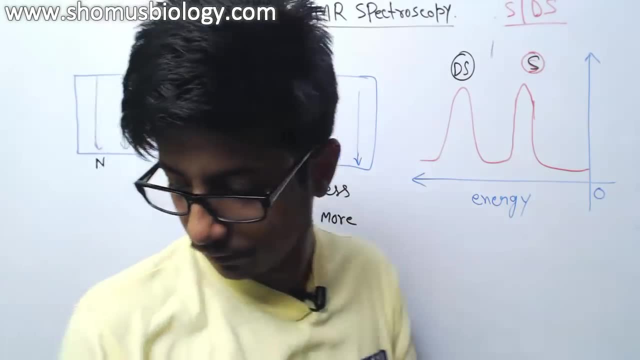 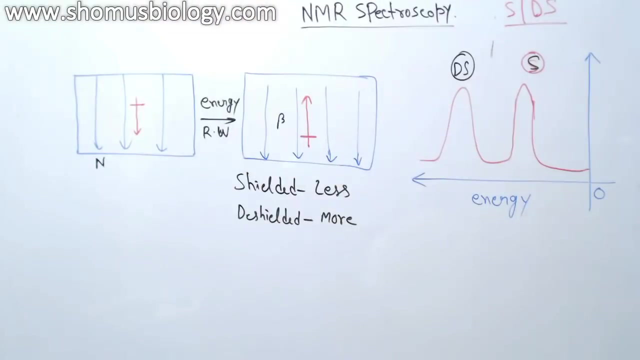 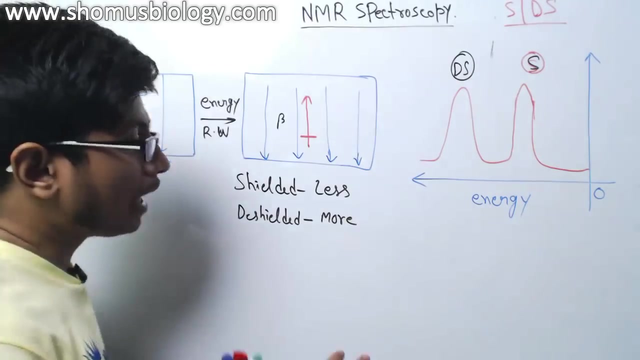 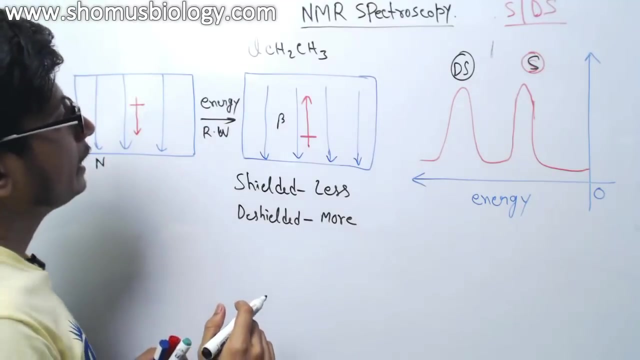 and how hydrogen is linked with other atoms plays the most important role about how it is going to determine the whole process and the structure of the chemical compound. Okay, so now let's see one chemical compound and how exactly NMR determines its structure. Okay, let's say the compound is CLCH2CH3. For example, now in this line we have a chemical 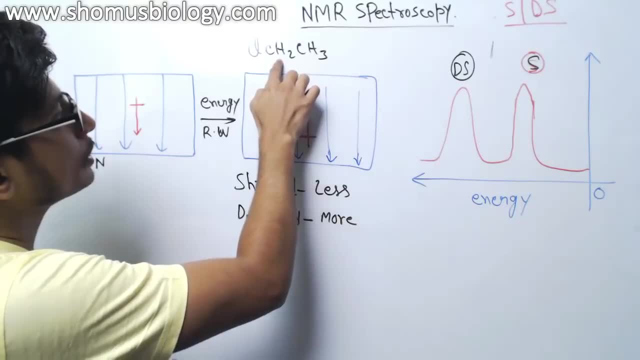 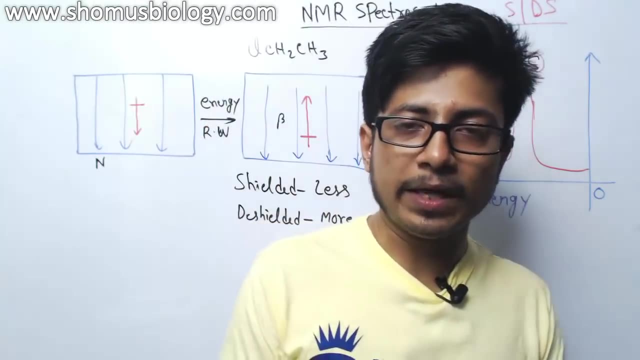 compound. In this compound you will see there are two hydrogen here and three hydrogen here, So there is a lot of hydrogen present there And actually, if you're talking about the organic chemistry and most of these organic compounds, they're hydrocarbon, So they're. 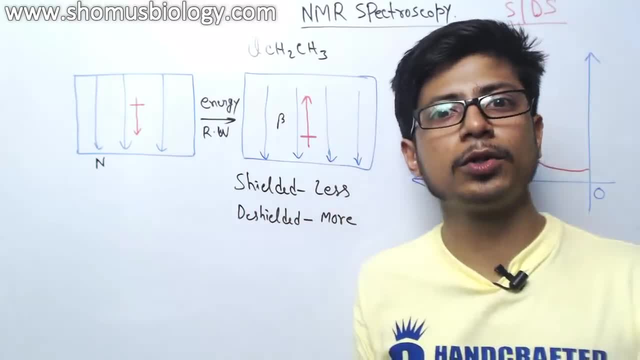 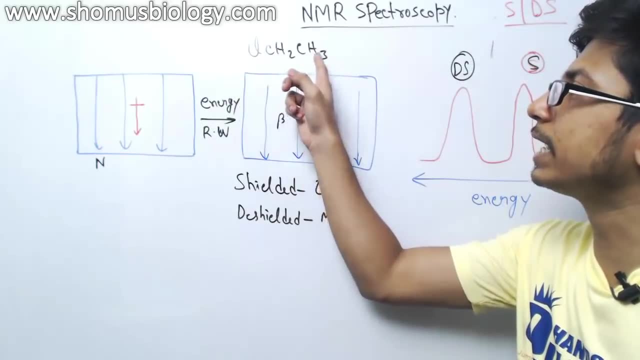 filled with carbon and hydrogen. So hydrogen is present in all those molecules And those hydrogen will be very beneficial for us to find out the exact arrangement of those atoms that forms that chemical compound. Okay, so now let's look at, in this case, 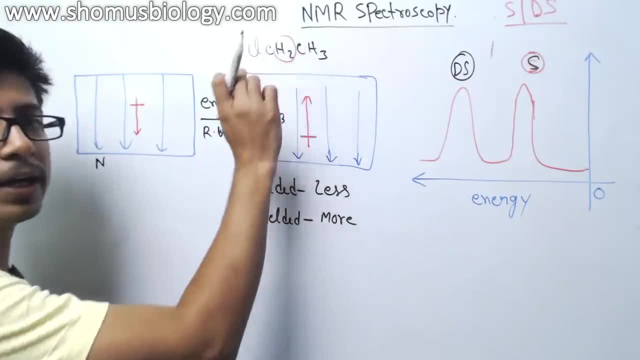 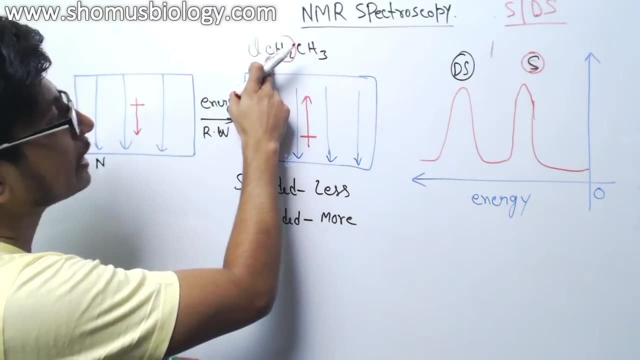 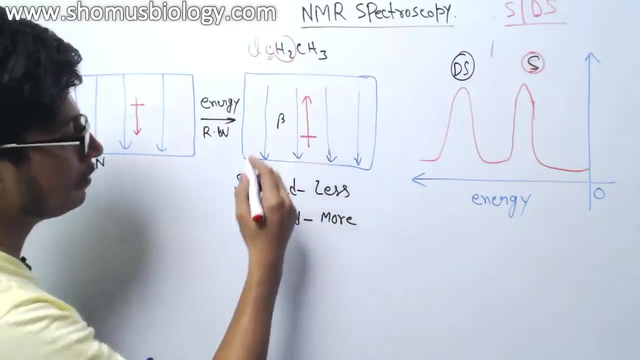 if you think of this hydrogen in the middle, let's say one hydrogen that is present here. Okay, so the hydrogen that is present and attached to the carbon. so the nearest attachment of nearest atom for the hydrogen here is this carbon. right, That means this hydrogen. let's 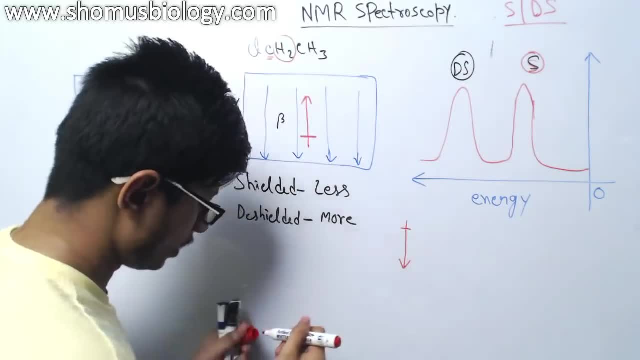 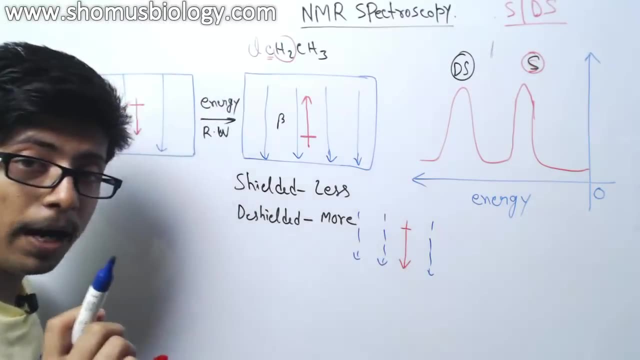 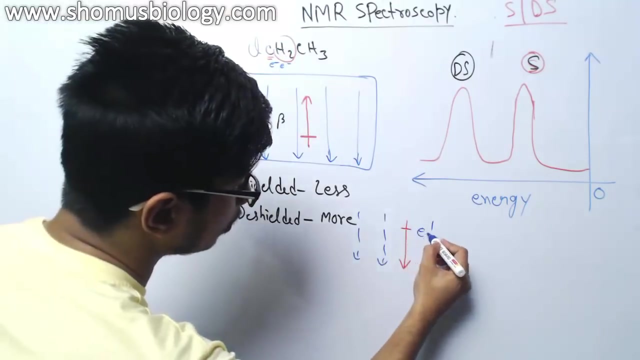 say: this is the hydrogen, it will try to behave like a magnet. it will be arranged according to the magnetic field. Let's say that, But, But, But. But. there is this electrons coming from the carbon, the nearby carbon. So there will be. 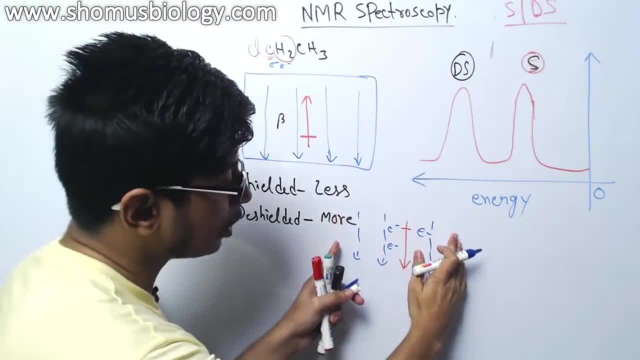 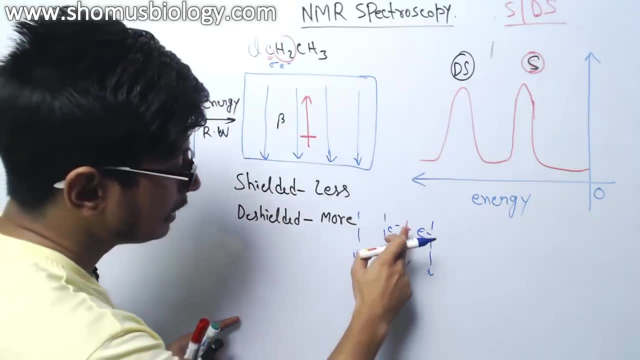 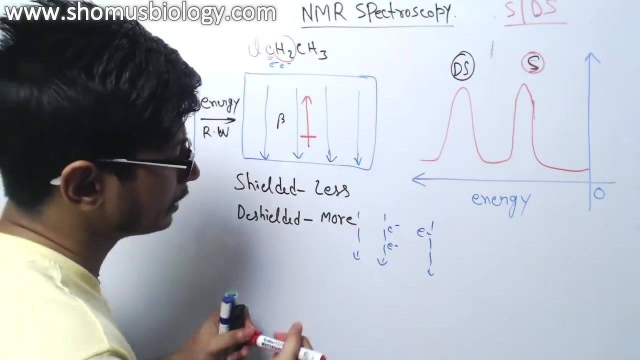 electrons from the nearby carbon. that will not allow the effect of the magnetic field that we apply in the NMR machine to this molecule. As a result, this hydrogen will not properly align with it will not properly align with this magnetic field because it is shielded. 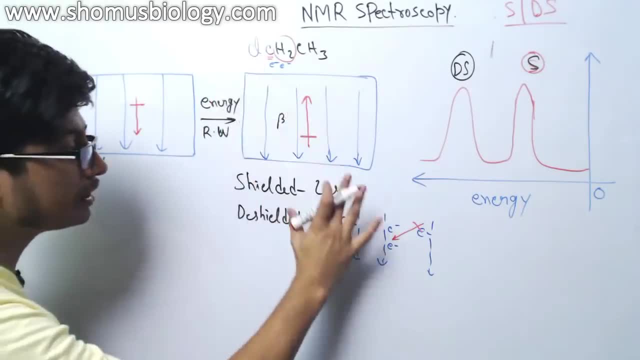 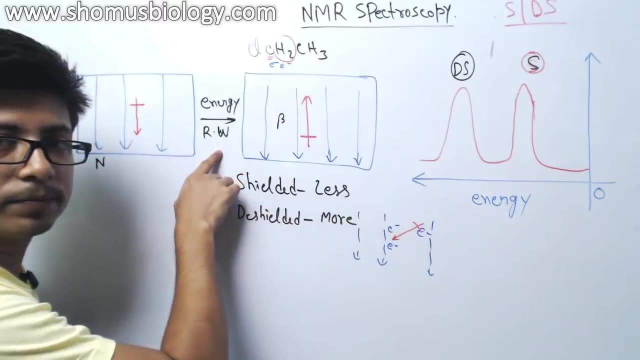 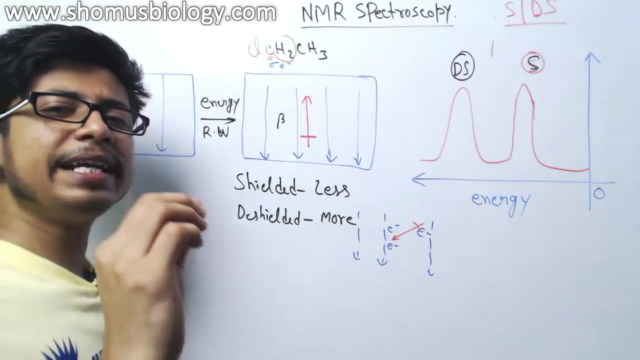 by the electrons coming from the nearby carbon. So this is a shielded situation. Now, if we put the radio wave light source, that will be acting as an energy to shift it to the beta spin state. we need very less energy because it's already shielded with electrons. 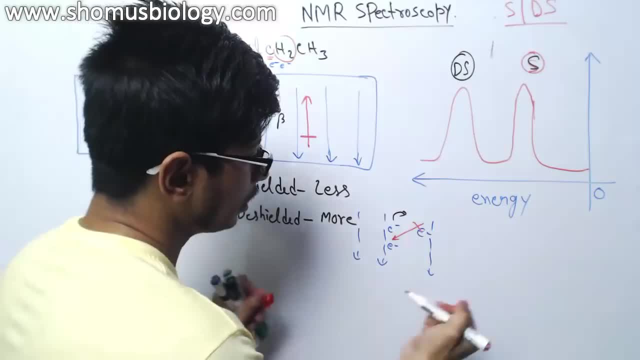 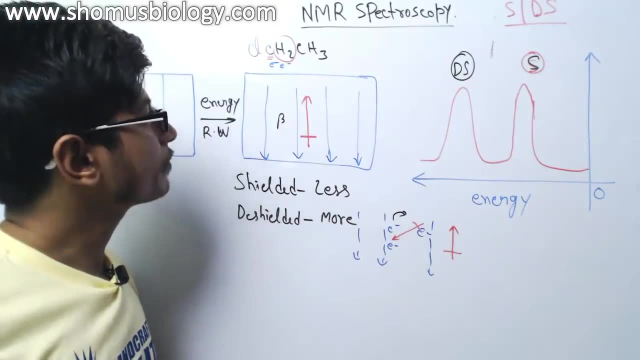 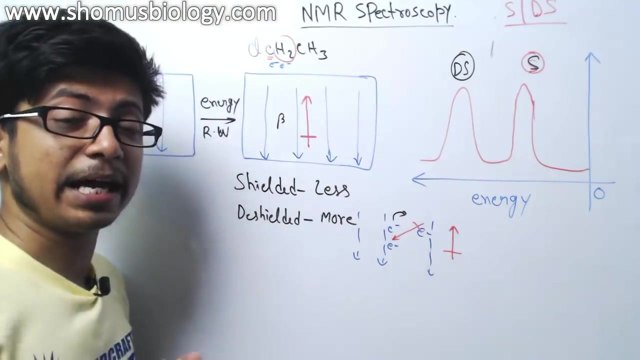 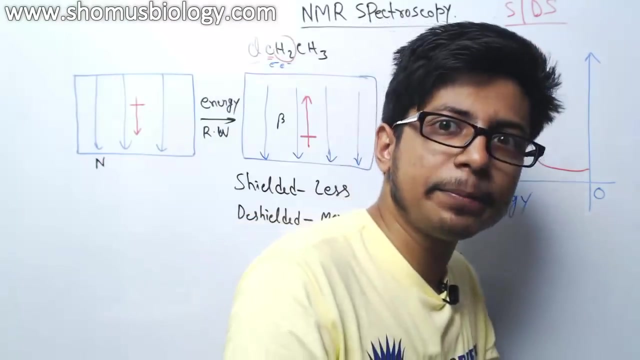 really less energy, to put it back to the structure, Right, So very, very less energy. But now let's think of this idea a little deep life. just think of this. carbon and hydrogen- you may think like that, but there is a chlorine present next to the. What does that mean? 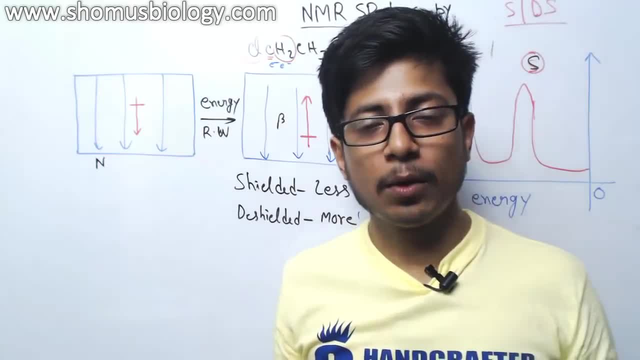 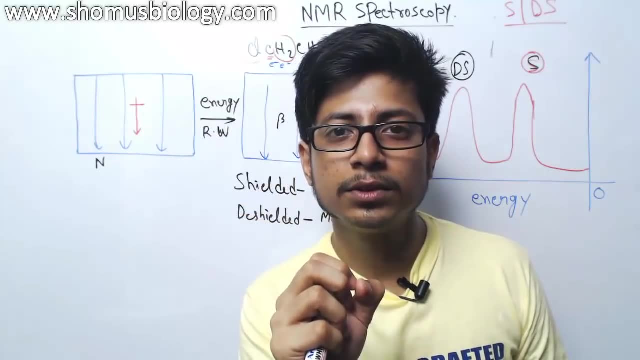 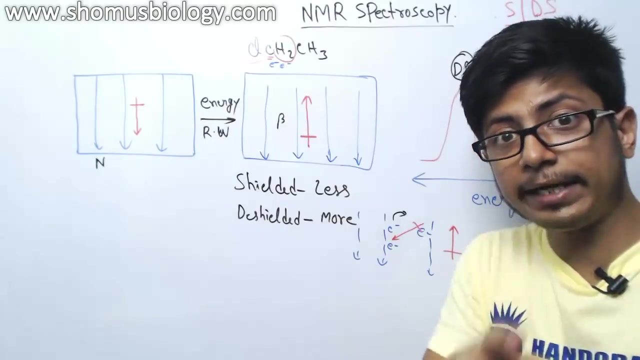 Chlorine has higher electro negativity. What electrolegitim 원 Lg electronegativity does electronegativity means chlorine have the affinity towards electron, So it will take all those electron towards itself from the carbon. So now the idea: electrons. 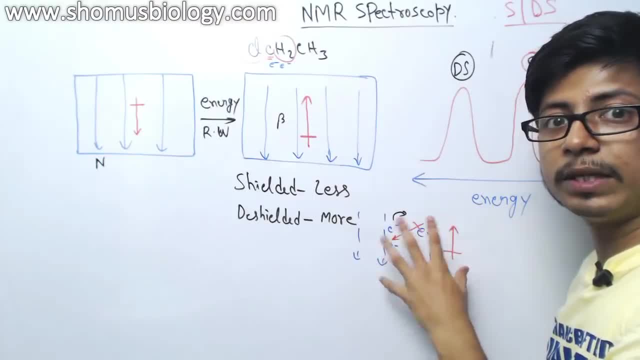 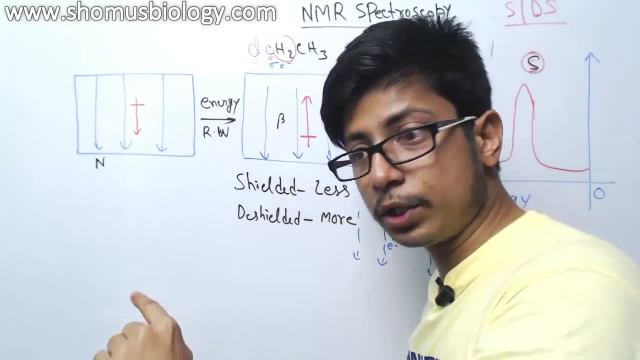 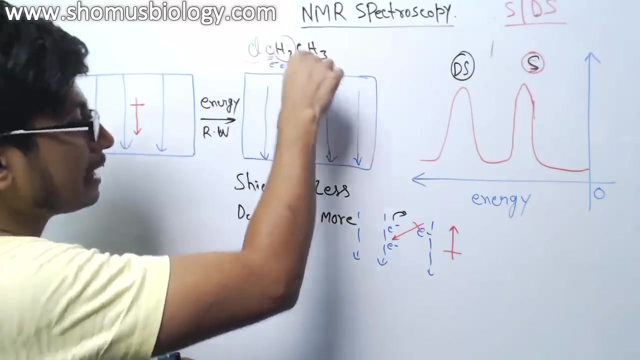 are surrounding this hydrogen, masking the effect of the magnetic field, But now, as chlorine is present very near to the carbon, it is dragging electron towards itself due to its electronegativity. As a result of that, as a result of that, this hydrogen is not properly. 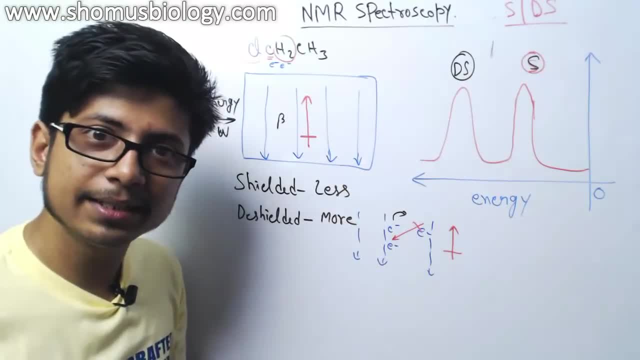 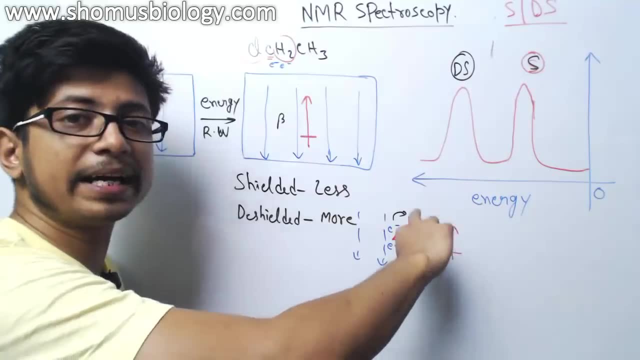 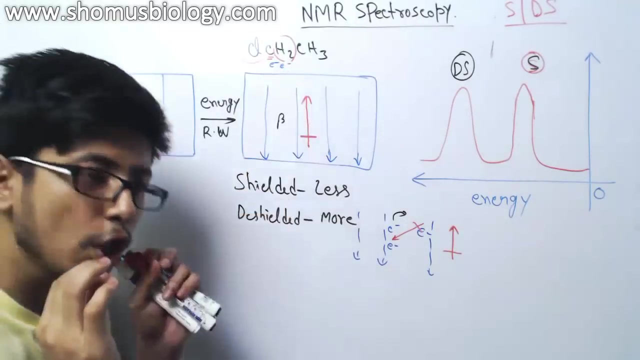 shielded, as it supposed to be right. If the chlorine is not present, then it should be seen shielded and we need less energy to feel to put it back in the beta spin state. But now, as chlorine is present nearby, it is taking the electrons. So now the hydrogen is not. 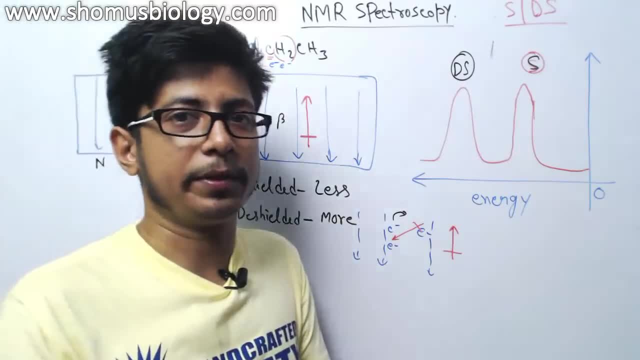 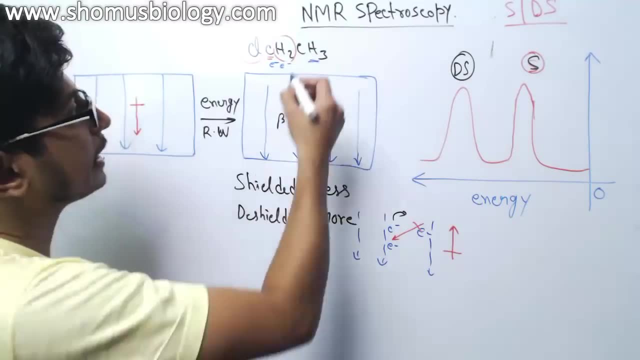 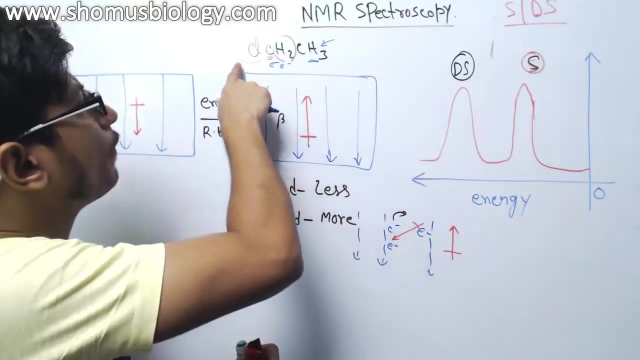 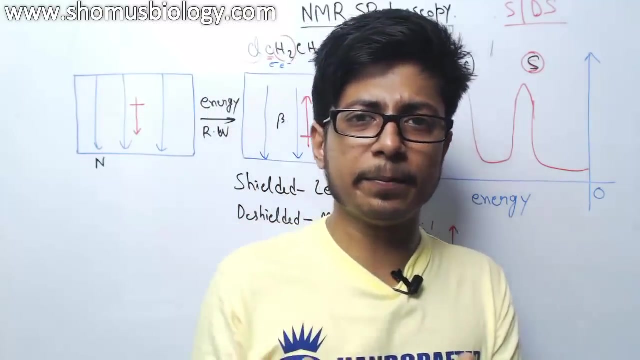 that shielded. So we need more energy, Reggie, to deal with it. take another hydrogen that is present here. That is this one, The second hydrogen here. there is no chlorine, no electronegative molecules nearby that longer is present, for that does that mean the electronegativity is a very nearby process. It's a very local. 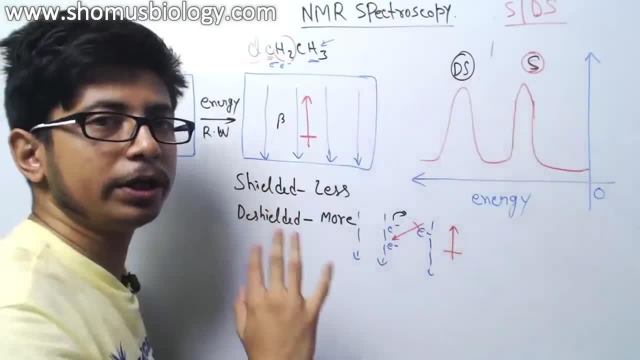 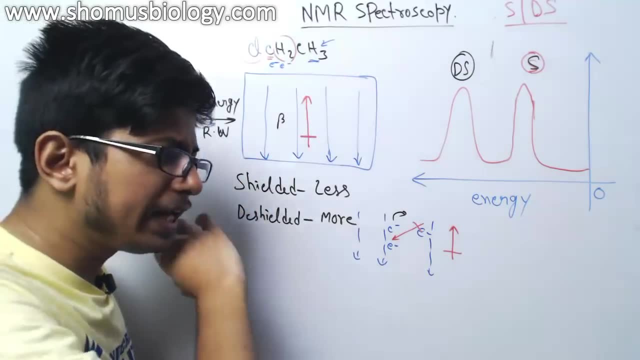 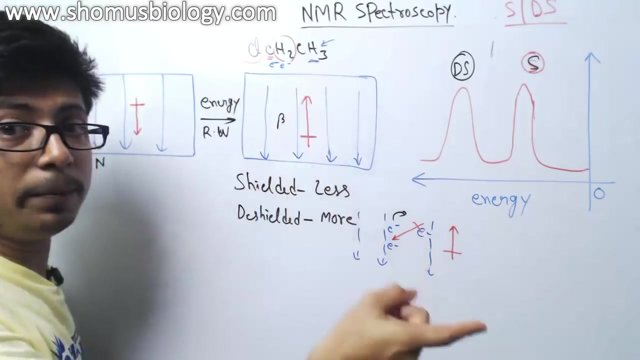 energy local process. It is not spread across the whole molecule, It's all It's across a specific region surrounding the chlorine. So this hydrogen do not have any impact of this electronegativity of the chlorine. that is far apart from it. So this hydrogen will. 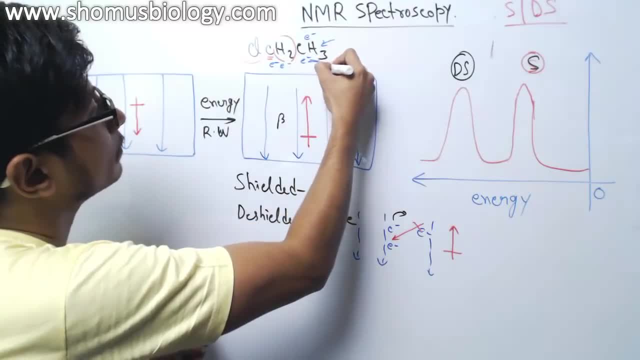 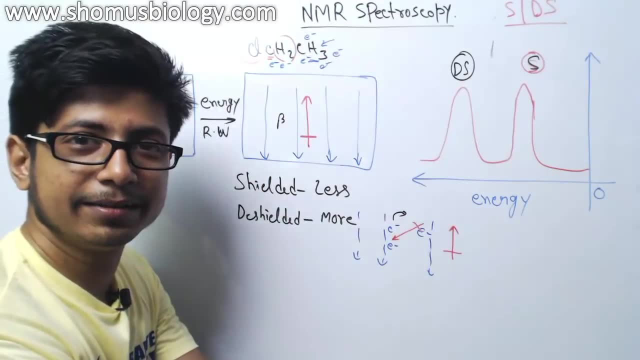 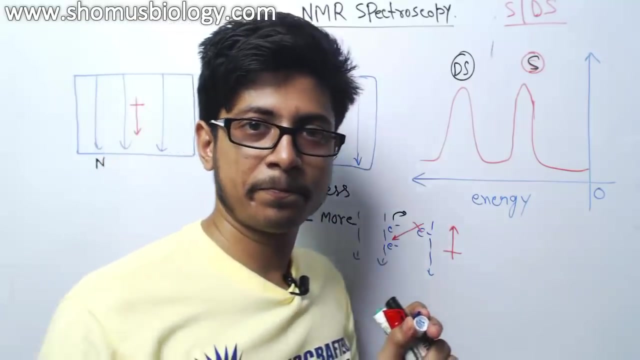 be shielded by all the electrons coming from the nearby carbon, because this hydrogen also have a nearby carbon right. So this hydrogen will be shielded by electrons, So we need less energy to shift it back to the beta spin state. So now, if we to take this to as a 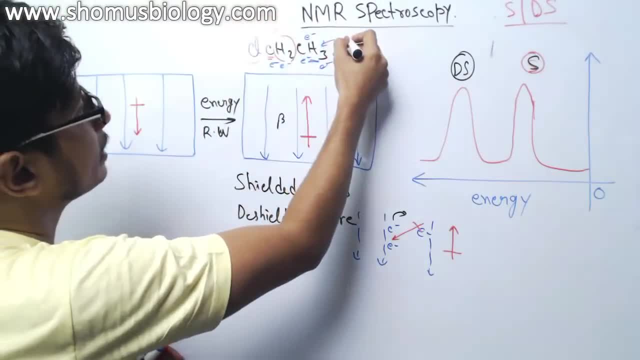 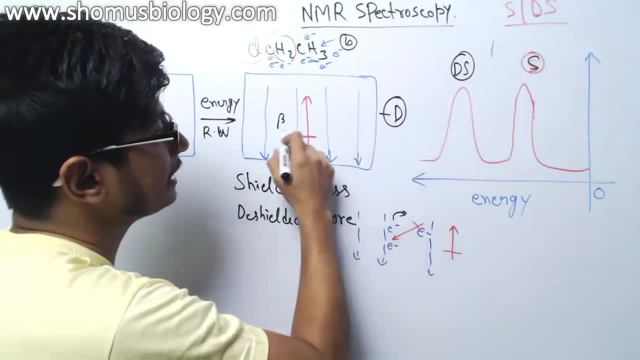 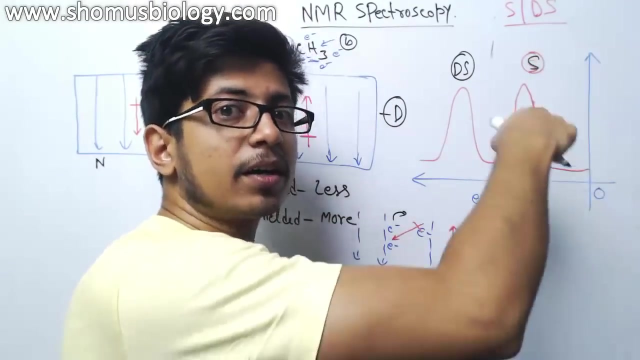 two population. this is this hydrogen as a, this hydrogen as B, what we can see in the actual peak that will be detected by the detector at the end of the NMR machine. If we look at this detector and if you look at the monitor screen, there'll be a, there'll be a graph. 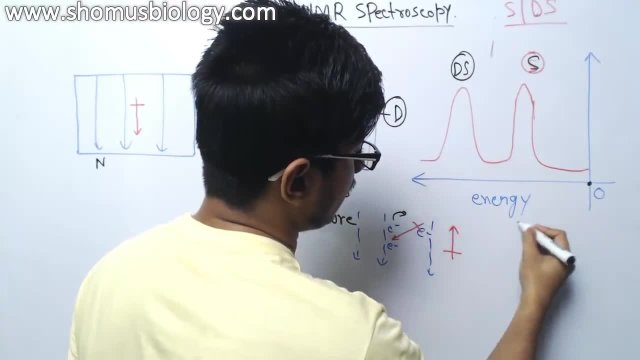 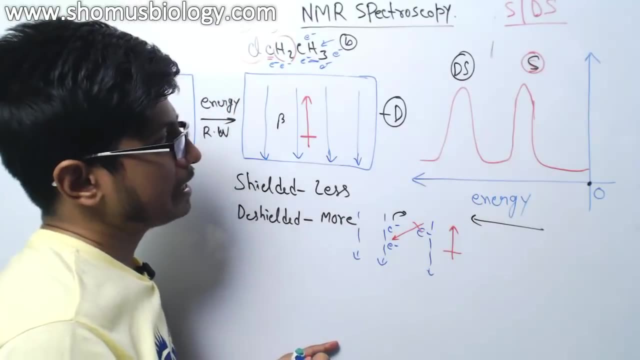 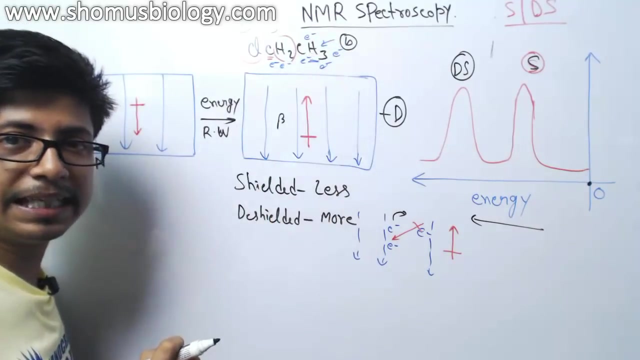 And that graph is telling us about the energy which starts from this point, And the energy is increasing in this direction, towards the arrow, And we have this intensity for there. So what? we will find out that the energy required for shifting this B hydrogen. 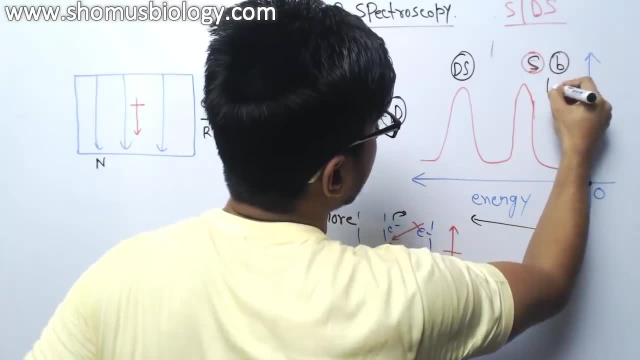 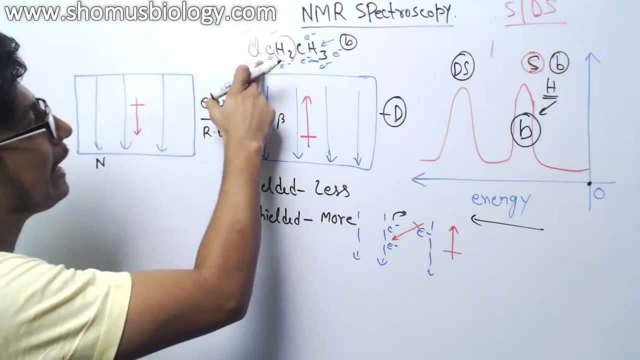 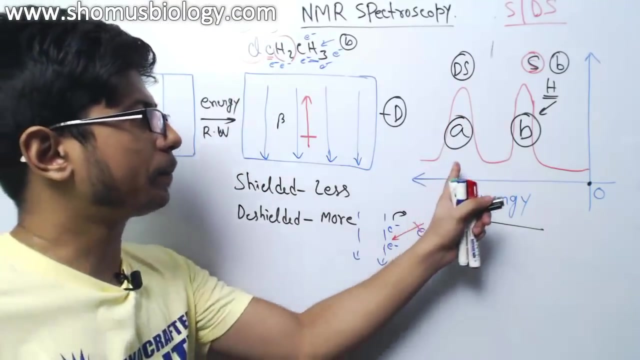 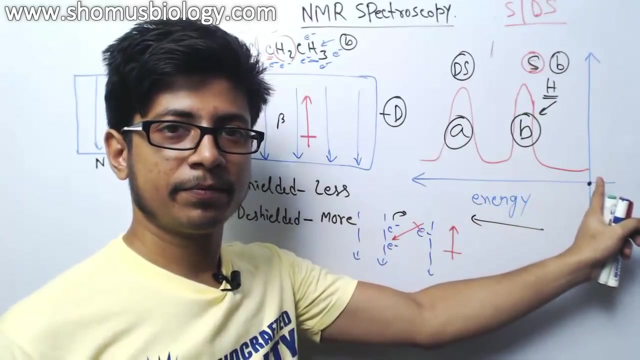 is less, So the B hydrogen will be present, representing the first peak. So this will be the peak for B. for a, this a hydrogen, there will be more energy required, So A will present every present in in the distant from the y axis here. So this is: 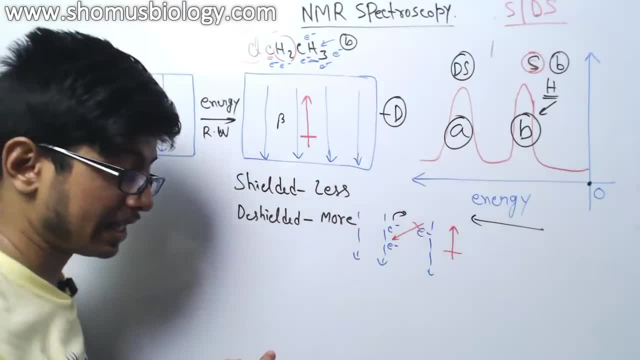 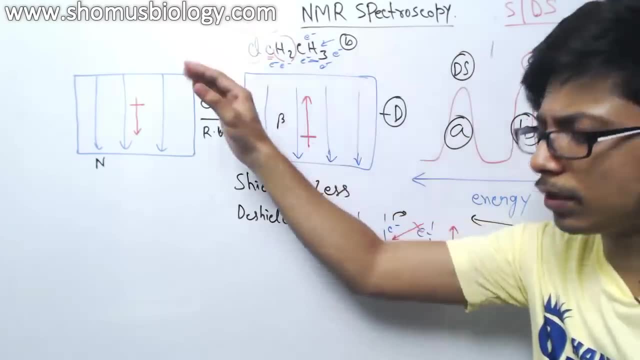 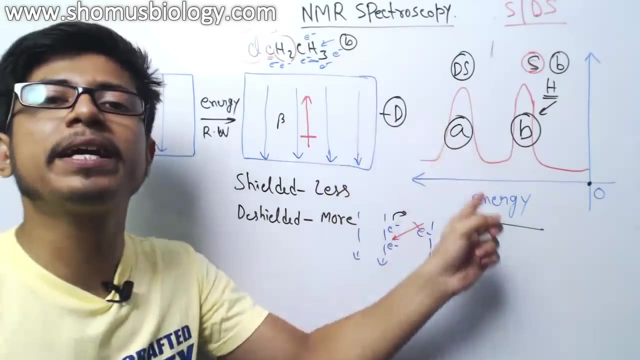 going to tell us about where exactly the B and A is present. Now, this is a very simple example to tell you what kind of situation it may arise. Now let's think about the presence of all those different special atoms surrounding the hydrogen. you will find a lot of peak. 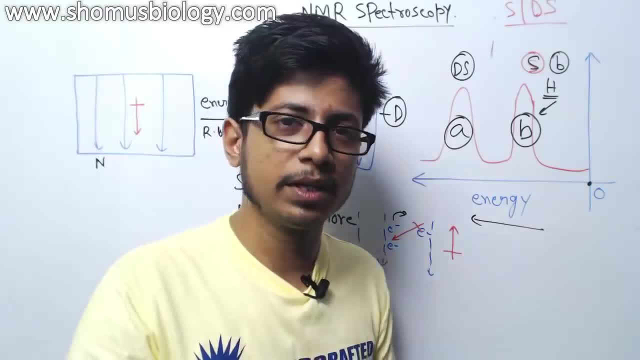 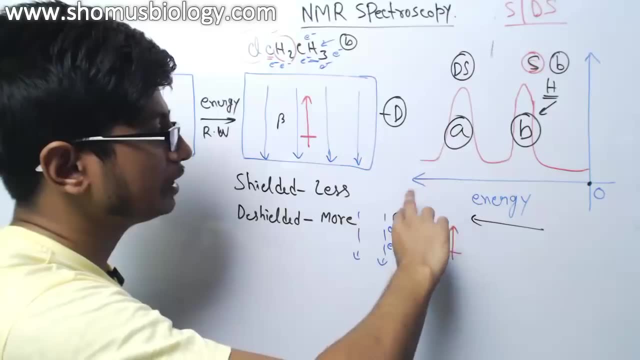 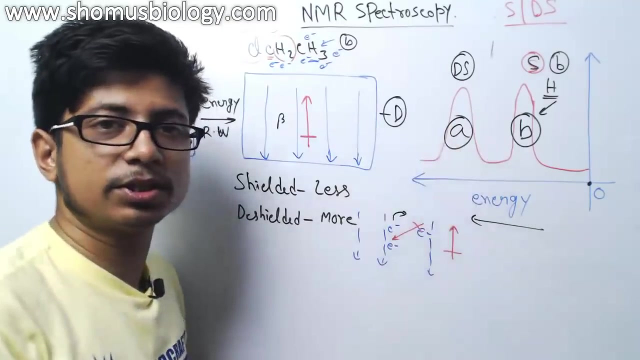 like that Huge amount of peak just going up and down. It's called the peak. peak is the graph, the point that is recorded due to this resonance energy, the energy that is required. So this resonance energy peak that will see it will be characteristic for different chemical compounds, For this compound. 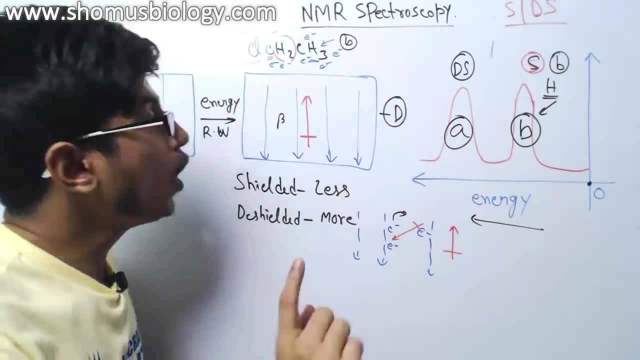 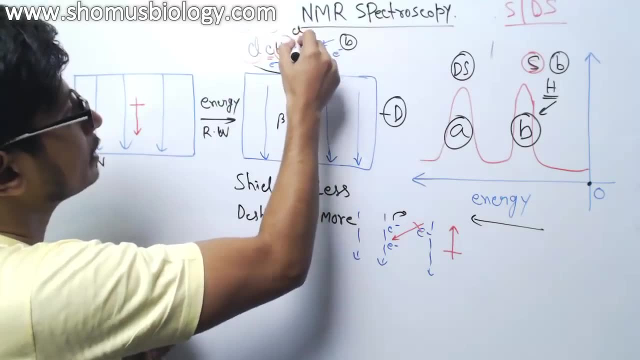 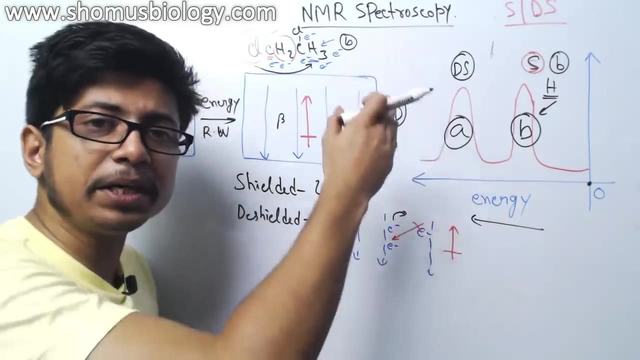 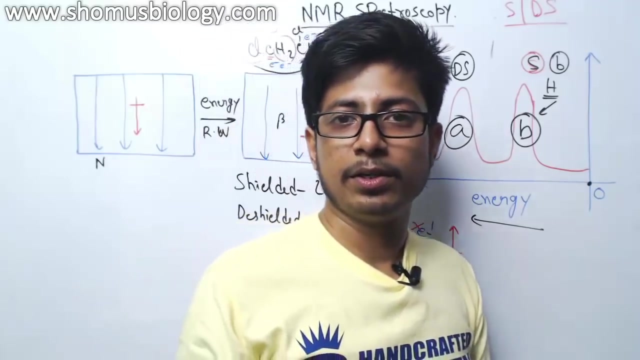 this is the character. for any other compound the character will be different. Or let's say, you take this chlorine from here simply and put it back next to this carbon. So this is going to be like a signature for a simple chemical compound. So once we analyze different